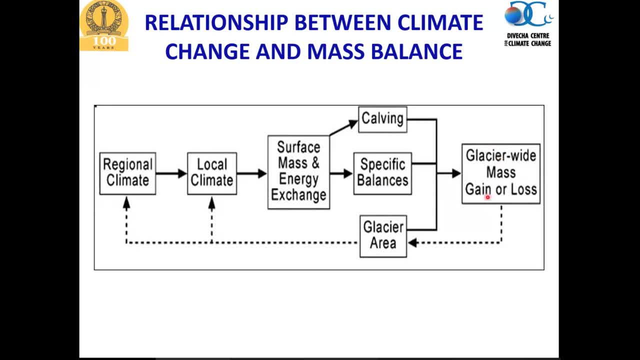 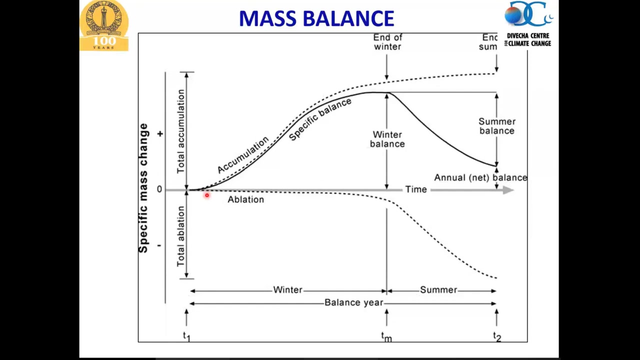 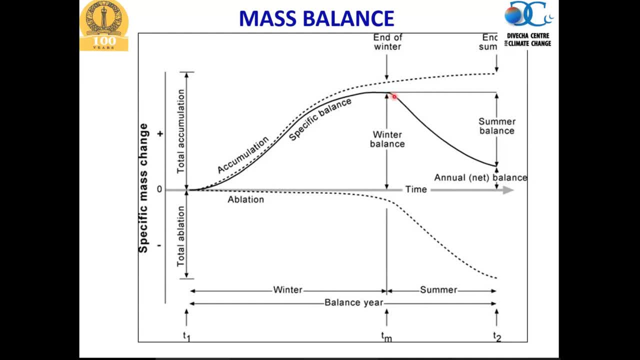 So then there is a total melting will start and the melting will. till the end of summer melting will take place. So what really happens is you have total accumulation like this and total melting like this. So this much difference is now annual net balance. Right, That is how the net So amount of snow left at the end of summer is a winter is a net balance. annual bank balance. 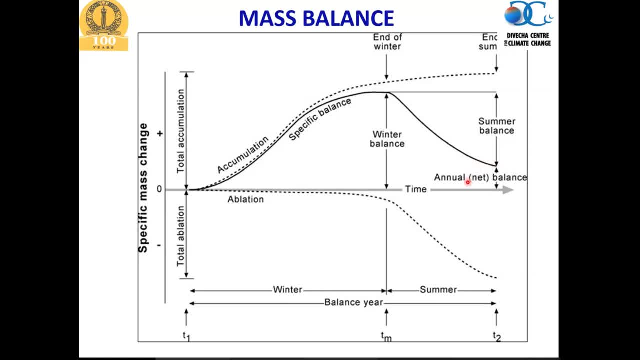 So You can look into two different ways into this one. You can also have a winter balance and also you can have a summer balance. So it is now many people will will do it separately. That means they like to call winter balance separately and summer balance separately. 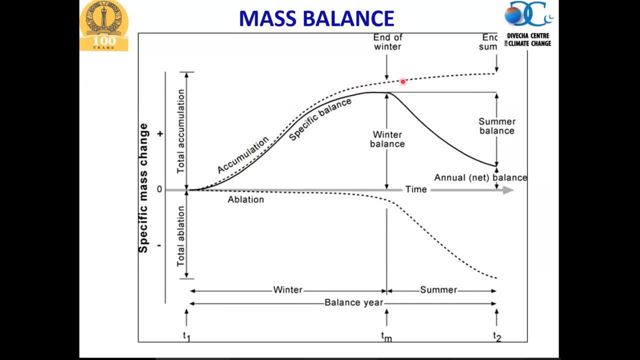 It also means, if you look into the accumulation, there is some snowfall is also going to take place in summer, So that is also. This curve is slightly going up, But ablation curve, this curve, you can see, and this is identical at this curve. 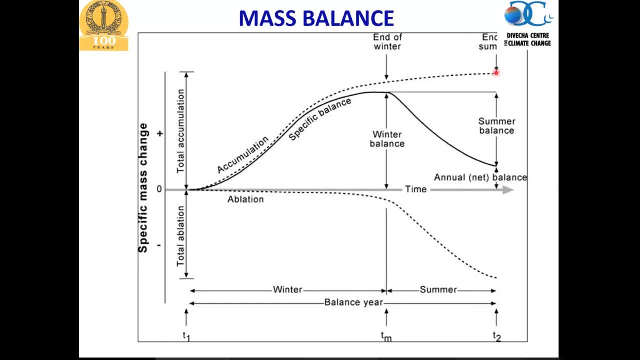 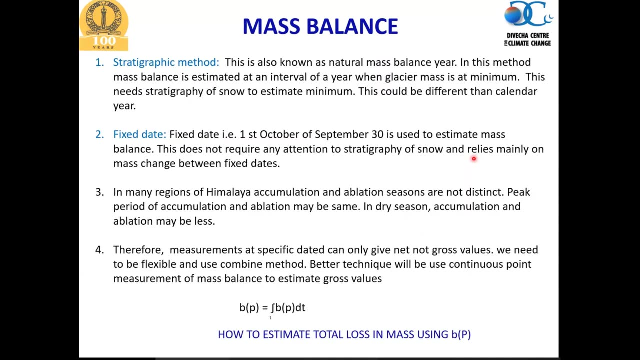 And then this is the left, or this is the end of summer, is the total accumulation, Then this is a summer balance And then this is a net, net, net balance. So we are generally interested in net balance. That is how it is curated. 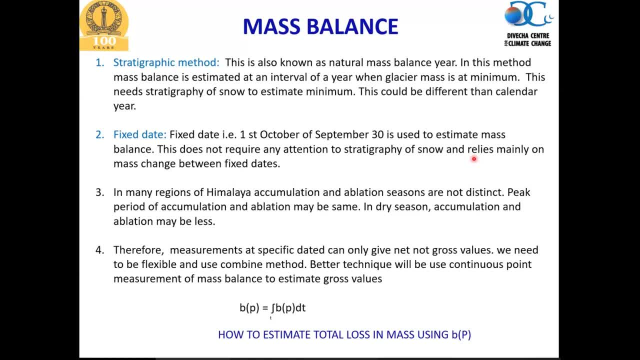 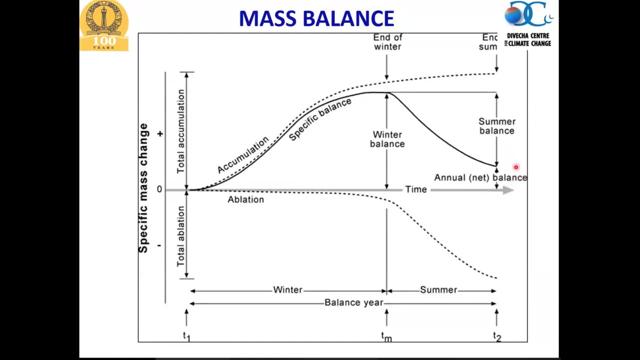 But there are really different methods. But if you are working in India and if you want to do mass balance, there are certain tricks or there are certain convention which is followed in India, So we need to understand that. So the mass balance, if you go into the previous term, what it means is you need to understand how much is the total annual net. 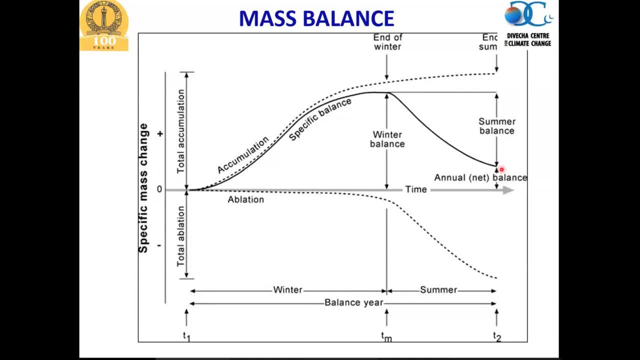 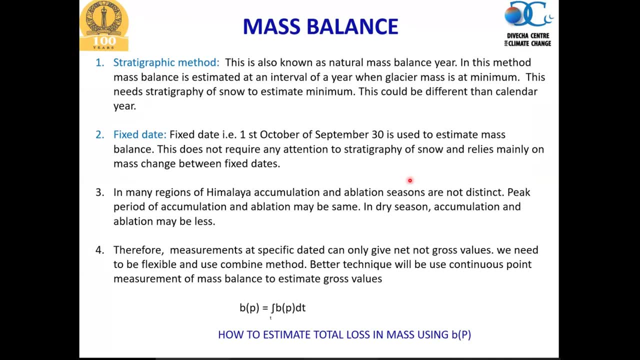 But if you go into next year, Then in order to identify what was the snow, what was this? No, because certainly in accumulation area you have a snow and then you have an ice, And so what happens is, at the end of summer, not entire snow is left. 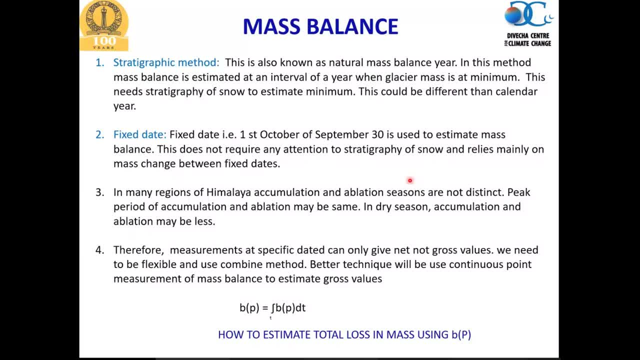 Some amount of snow is remains there And then there is a fresh snowfall. So if you next year when you go and you want to know how much is the accumulation, Why accumulation you need, you should have ability to identify where was the last year's snow layer. 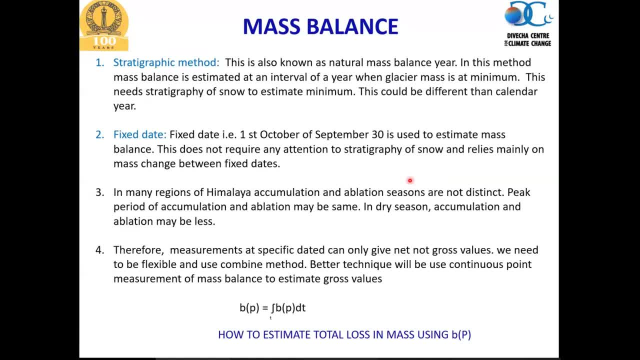 and from there onward you can say this year's accumulation. so stratigraphic method is. generally this is known as natural mass balance method. in this method mass balance is stable and at the interval of year when glacier mass is at minimum- and this needs stratigraphy of snow to estimate- 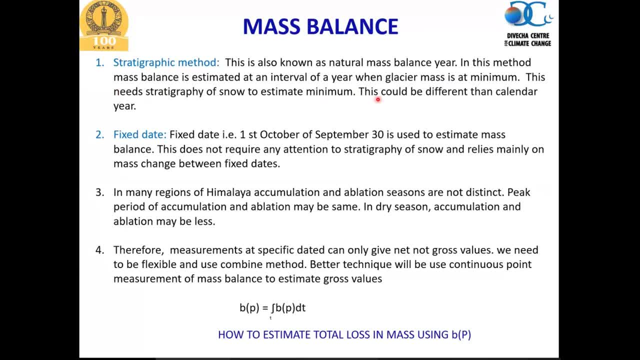 minimum. this could be different than calendar year. so what it means is that you, uh, you identify last year's, last year of the snowpack and how much it is accumulated in this year. on that you estimate and, however, this could be different than calendar year, essentially because every year snowfall is not going to arrive on exact date. 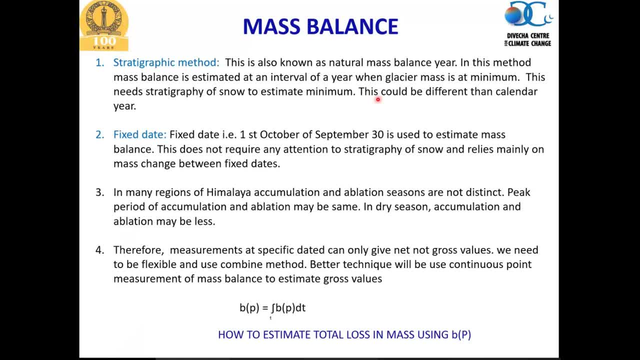 snowfall is going to arrive on exact date. snowfall is going to arrive on exact date to arrive depending upon various parameters. so the one year it could be in end of September, sometime even in middle of August you can have a heavy snowfall. so sometime it you may not have snowfall even till the end of October. so 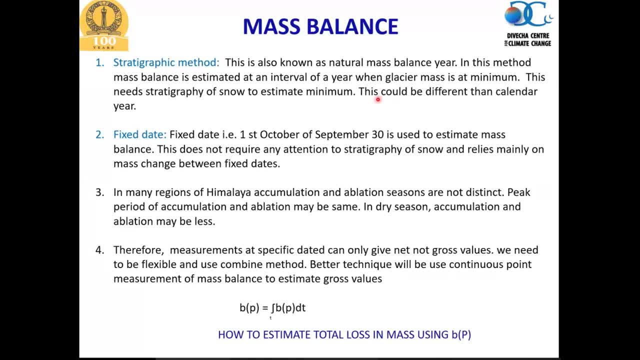 it will depend upon then. then how much is where snow is going to come, so this will be different than calendar year. however, India, most of the, it is usually fixed date, that is, you take it from 1st October to September 30th. why it is done. 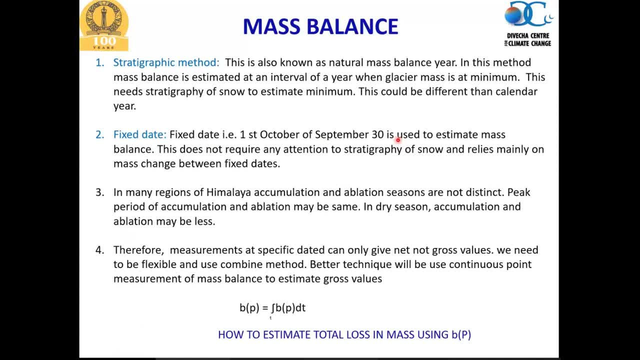 this is basically done by geological survey of India way back in 30s and this fixed date this year, 1st October to 30th October, is used to estimate the barn colors, and this does not require any attention to stratigraphy of snow and relies main on mass balance between. 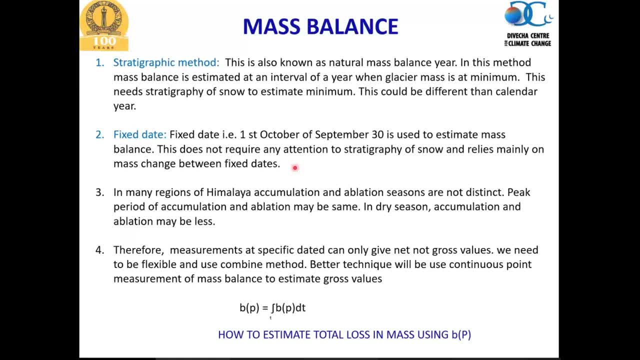 the fixed date. so if there is a heavy snowfall in the in the in the September, it will go into this year's mass balance and it will not go to next year's mass balance. so if you have a consistent record over a long period of time, it 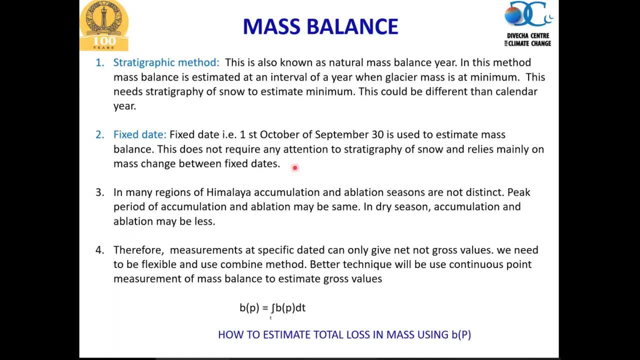 really averages it out and you get the some estimates of mass balance. you can see that it is very important to have a consistent record of a long period of time. it really averages it out and you get the some estimates of mass balance. in addition to that, in many regions of Himalaya, accumulation and ablation. 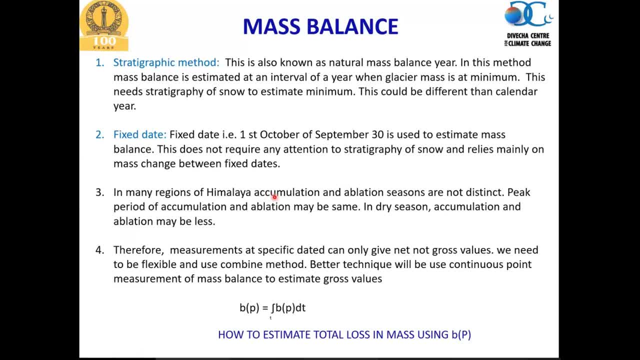 seasons are not distinct. peak period of accumulation and ablation may be same. so this is another issue which you will face is say, if you go into the Sikkim, then there is no, it is more like a Sikkim or Arunachal Pradesh or Bhutan. you have more like a 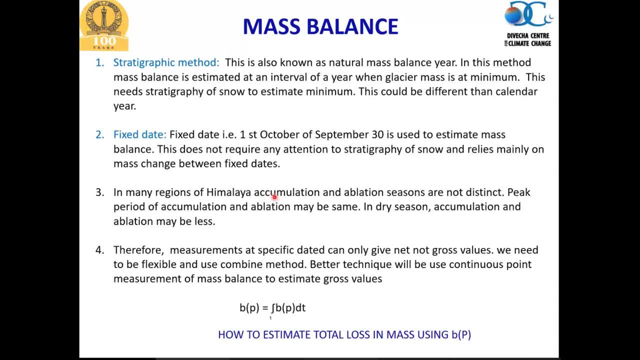 maritime climate. that means there is a continuous, throughout the year you are likely to get snowfall and throughout the year you are likely to melt it, and you have predominantly a lot of snow in summer and there is also ablation in summer, and therefore the peak of period of ablation and ablation may be same. 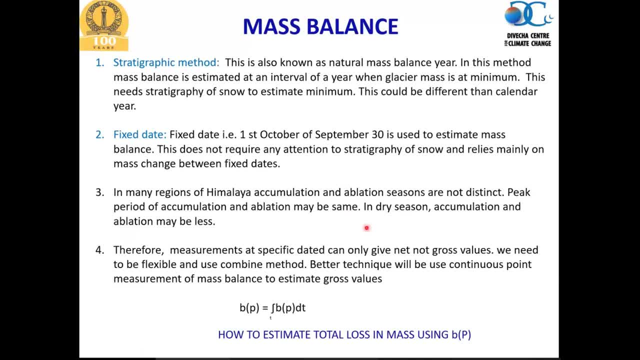 that is another issue. in dry season, accumulation ablation may be less, so you have to be a little bit more innovative in using the fixed date method. remember the fixed date method is predominantly used in Western Himalayas, at that time when Geological Survey of India started there. 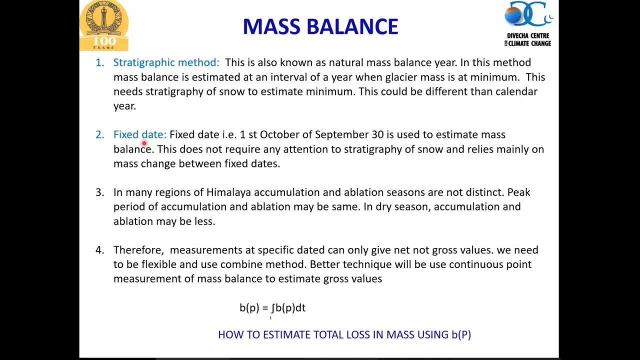 was very little work in Sikkim, so it is predominantly done in Western Himalaya. so therefore measurement of specific date can only give net and not the gross values. what it means is gross values and net values. you should understand. net means at the end how much it remains. gross means you have accumulation and ablation. 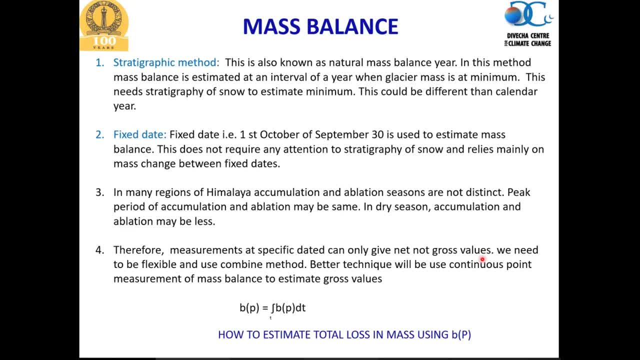 you have account for all that. that means throughout the summer, you know how much is accumulated and you know throughout the summer how much is ablated, and that will provide you it. so you have continuous record of snow accumulation and ablation and this give you gross value. net value is: you don't know. 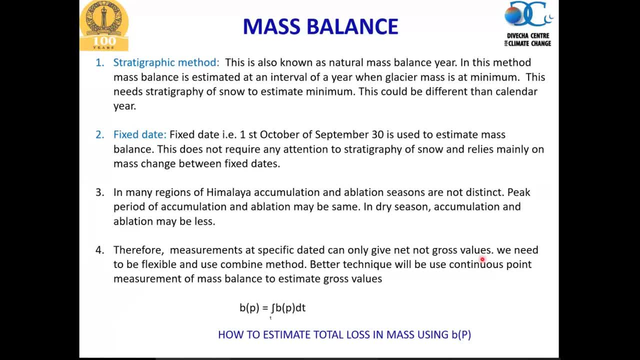 in intervening period how much it is snow and how much it is melted, but you know at the end how much is remained. therefore it is called network. we need to be flexible and use combination of method. so there is nothing which you can do depending upon region and climate. you have little bit flexible and make sure that you use the 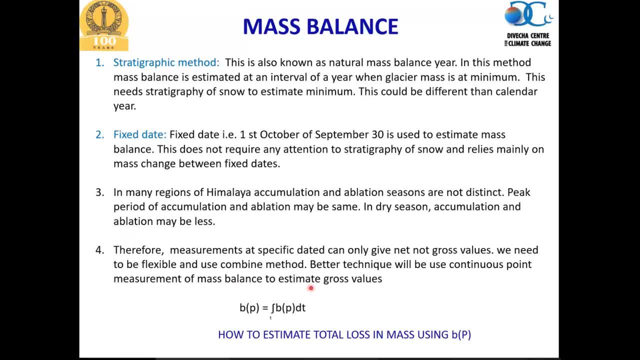 combination of method, better technique will be used: continuous measurement of mass balance to estimate. estimate the gross value, if you can do it, essentially because, remember, mass balance is a major exercises. you can't access glacier easily in winter time, when it is a thick blanket of snow and the regions are completely so you have to have some estimate. so this is 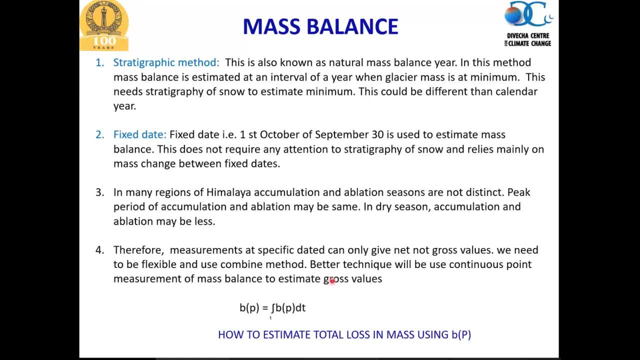 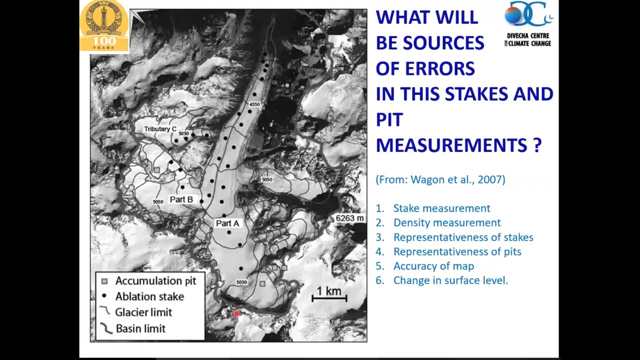 a. if you have, if you want to get gross values, then you have integration, mass loss over a period of time and you get. you get the total value of mass loss, pp. so it is indeed, you know, possible for us to do that in this way. so it is important for us to understand how we do the glacial mass balance. 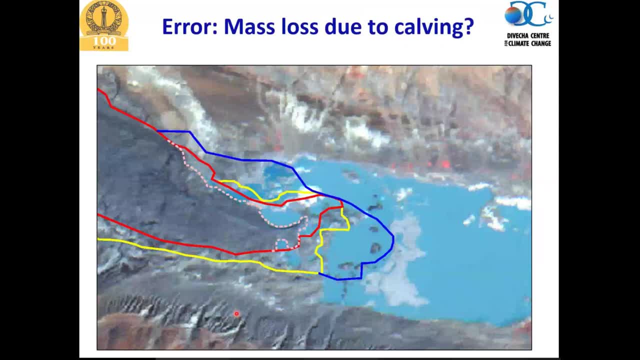 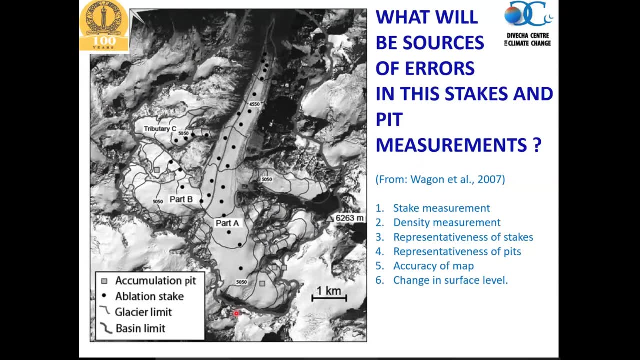 and one of the conventional method to estimate the glacial mass balance is a glaciological method. that means you go into the ground and try and get the mass loss by using certain measurements in order to do that glacial mass balance. why? what predominantly you do is you. you put the stakes, you 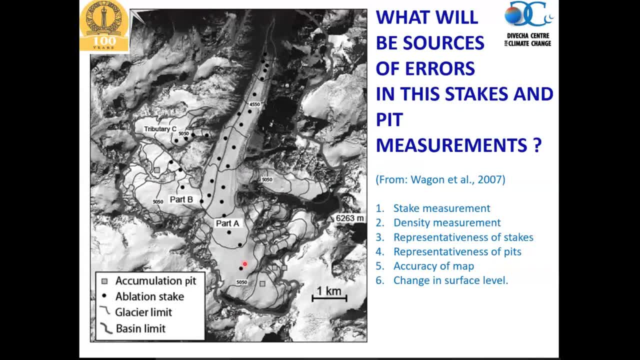 this is a chota shigri glacier in himachal pradesh, and this work is done by the glacial mass balance was done Magnum and other man, and thus so you can see here this is the ablation area. certain regions have very debris cover and then you put the stakes. 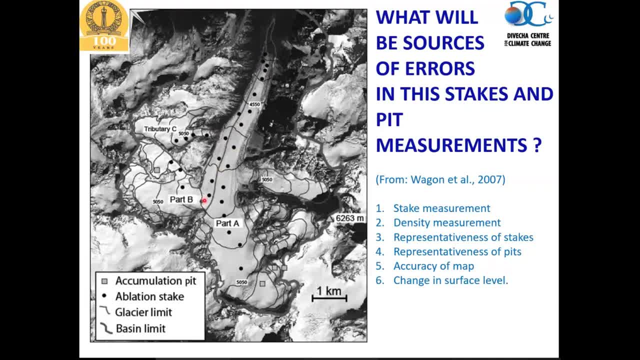 like this: numerous stakes in various altitudes on. this is a contour, so you get the this region is on to is the elevation zone, and each elevation zone you get the, you get put the stakes. stakes are nothing but the vertical, vertical pole. you drill it and put it inside the ice, and this is done. 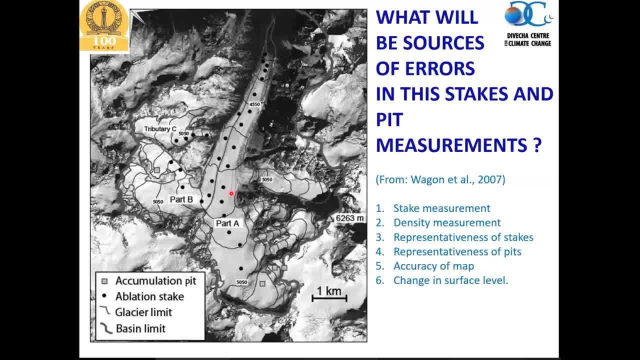 predominantly in ablation area where ice is exposed on the surface. and then you mark and you go there at the end of summer and that you know that in conventionally it is 31st September, so you go before that. you measure the, you mark the glacial surface. 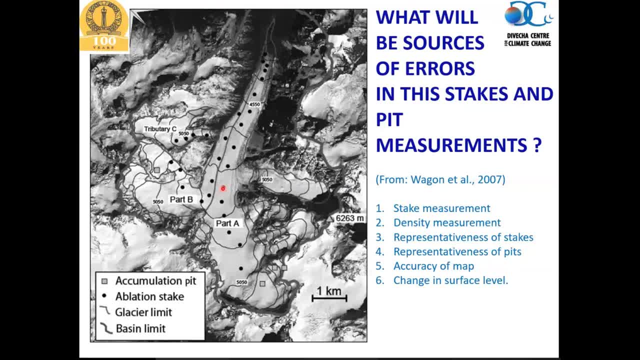 you go next year and again you take out. you find out from that distance how much is glacier, glacier, our surface is lower or melted, and you get a mean by knowing it in different altitude zone. you have then one value for each altitude zone and you get the total meant. 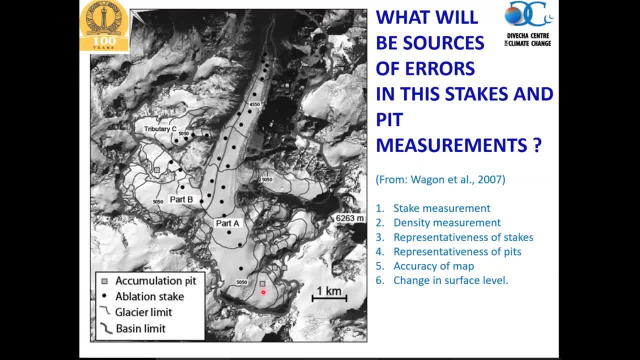 you also go into the accumulation area over here. you can see and they square, you create, you make it quit. that means you did this, not back and make a pit of snow. and then you measure how much is the thickness of snow at different interval. you measure be, you measure the density so you get the total mass of ice, so you 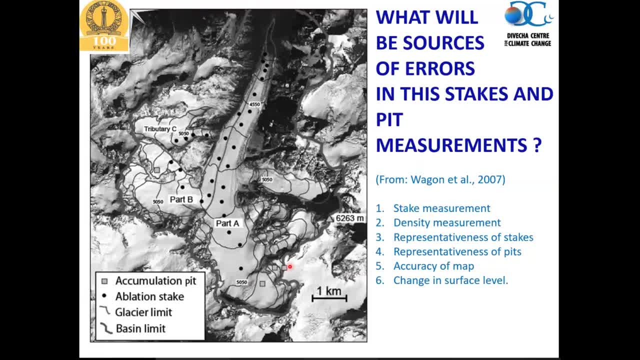 do it places. however, there are certain issues. so at the end you have how much is the total accumulation of snow at the total ablation of snow at the end and you get the mass loss. so that is how the conventional glaciological methods is done. but difficulty comes in this, even though you put lot of stakes there, since 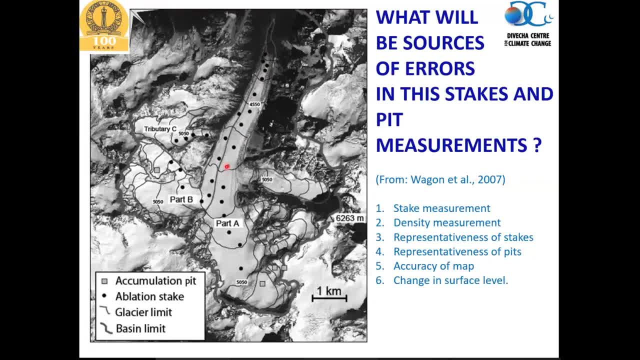 glaciers are moving. it is melting. by the time you reach there, many of the glaciers stakes will be nearly fallen, and that is a practical issue, and because of that, what happens is you may not able to get some here. some stakes will be fallen. they are randomly fallen and there may not be sufficient data in 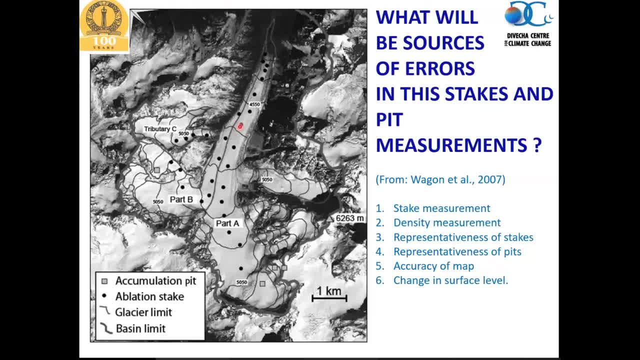 each altitude zone and can add some error into this- the piece are generally- you can add some error into this- the piece are generally few and far between, essentially because this requires the enormous human effort. you can remember staying about 5,000 meter for we, if you want to do one pit. 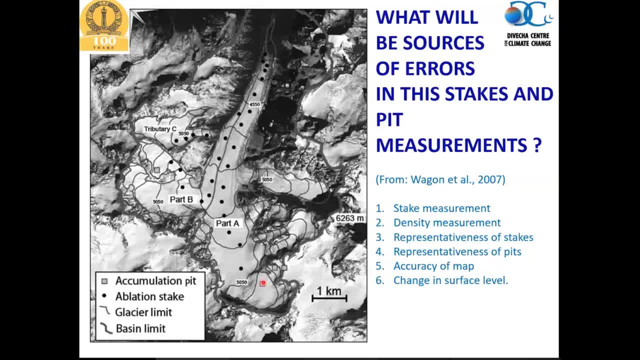 you will require one day at least to do the pit and do it. it is very physically demanding work and because of that very few pits are taken and they may or may not represent entire geographical area, which were talking because we are also. we are also discussing the geological area, which we are talking because we are also. 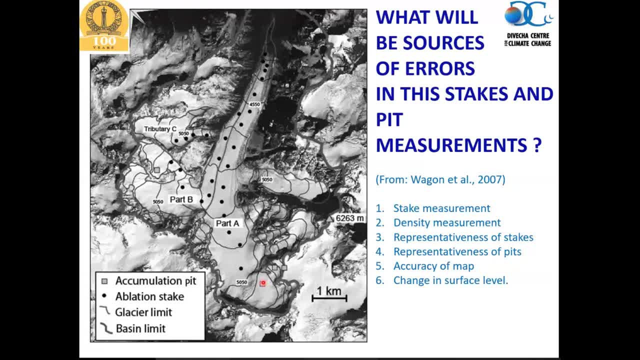 discussing the geological area, which we are also discussing the geological area, because we are also discussing the geological area, which we are also discussing the geological area, which we are also discussing about the avalanches accumulation, so the about the avalanches accumulation, so the about the avalanches accumulation, so the deposition of snow, fire, snow on glacier. 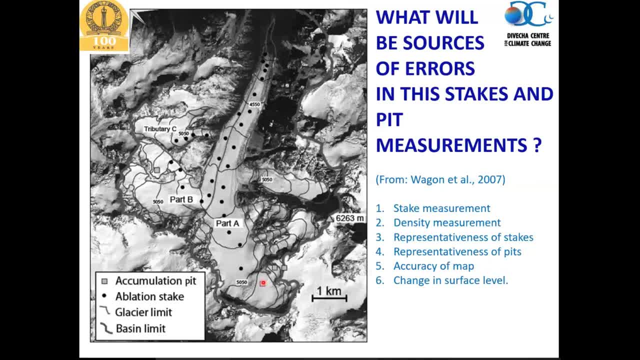 deposition of snow fire. snow on glacier. deposition of snow fire. snow on glacier may not be, may not be uniform and the may not be may not be uniform and the may not be may not be uniform, and the special variability of snowpack is not. special variability of snowpack is not. 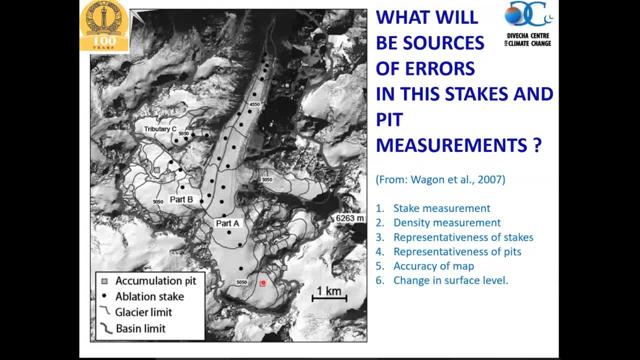 special variability of snowpack is not properly detected by few pits and properly detected by few pits and properly detected by few pits, and creating problem. then addition to that, creating problem. then addition to that, creating problem. then addition to that, there is a problem on accuracy of maps. 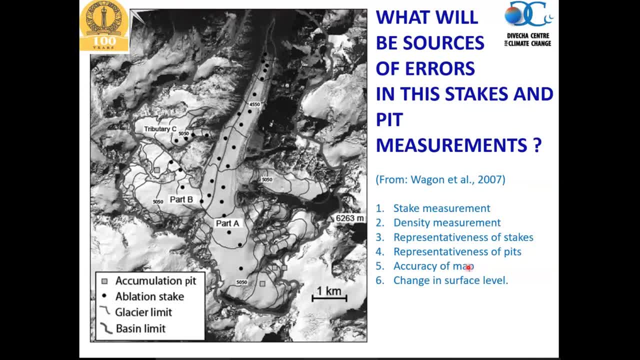 there is a problem on accuracy of maps. there is a problem on accuracy of maps because most of the time maps are over, because most of the time maps are over, because most of the time maps are over, so it's area also changes and change in, so it's area also changes and change in. 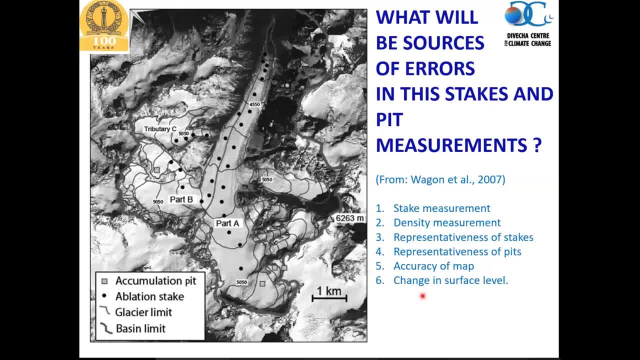 so it's area also changes, and change in surface elevation can also cause some. surface elevation can also cause some. surface elevation can also cause some error. so there are certain errors but error. so there are certain errors but error. so there are certain errors, but historically people have not done error. 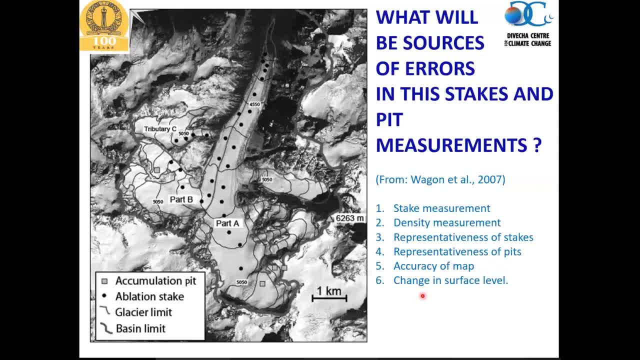 historically people have not done error. historically people have not done error: analysis in in a conventional method and analysis in in a conventional method and analysis in in a conventional method and glaciological method. but then I think glaciological method, but then I think glaciological method, but then I think around year 2004 and 5, many, some of us 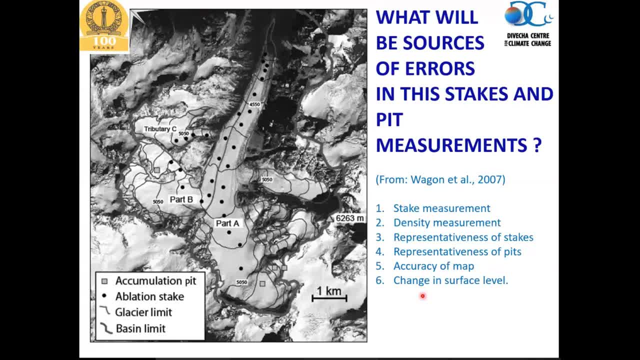 around year 2004 and 5. many, some of us around year 2004 and 5. many, some of us have insisted that you should have this, have insisted that you should have this, have insisted that you should have this error, error, error estimates, and we started to reject the. 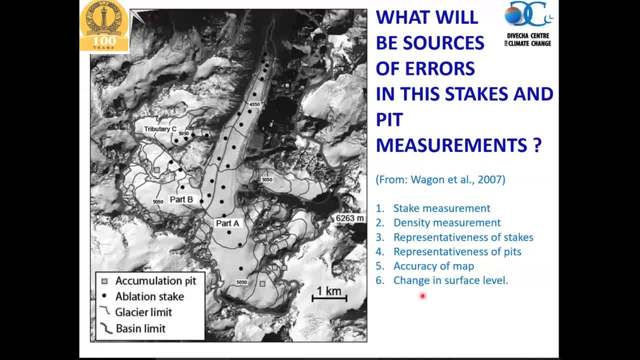 estimates and we started to reject the estimates and we started to reject the paper. then only some of them have paper. then only some of them have paper. then only some of them have started to put error into the. this started to put error into the. this started to put error into the this analysis. so this is also enough there. 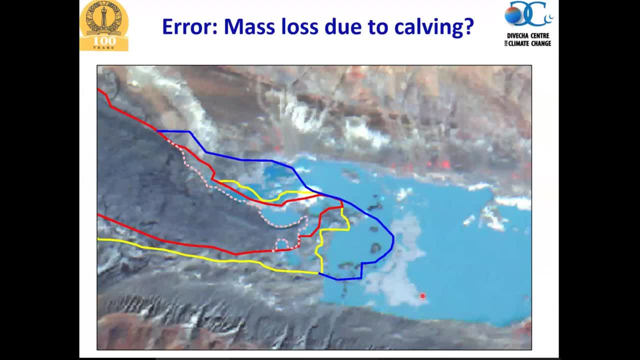 analysis. so this is also enough there. analysis, so this is also enough there. another issue in this method is mass. another issue in this method is mass. another issue in this method is mass loss. due to call me so what you really loss. due to call me so what you really. 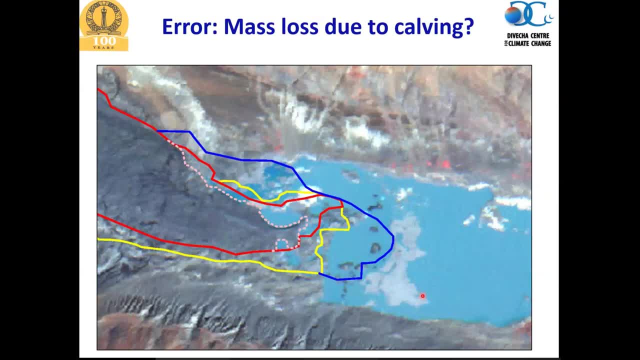 loss due to call me. so what you really look into this is: this is a chota. this look into this is this is a chota. this look into this is this is a chota. this is a some of the top of glacier in is a some of the top of glacier in. 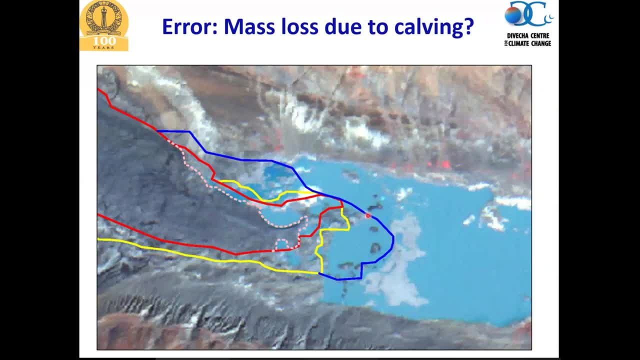 is a some of the top of glacier in Himachal Pradesh and you can see these Himachal Pradesh and you can see these Himachal Pradesh and you can see these eyes, which is completely detached from eyes, which is completely detached from eyes, which is completely detached from main body. so you, if you consider, 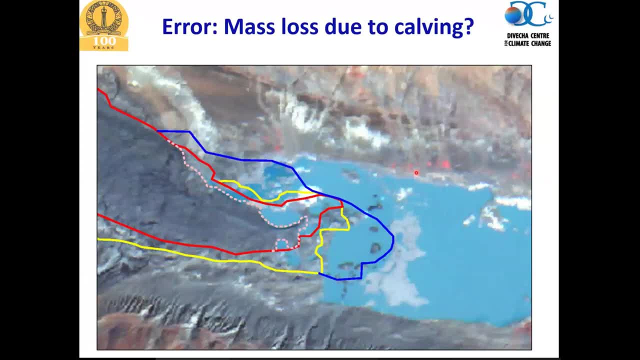 main body. so you, if you consider main body, so you, if you consider whatever loss is called because of the, whatever loss is called because of the, whatever loss is called because of the carving is not accounted in the stake. carving is not accounted in the stake. carving is not accounted in the stake and pitch method making this is adding: 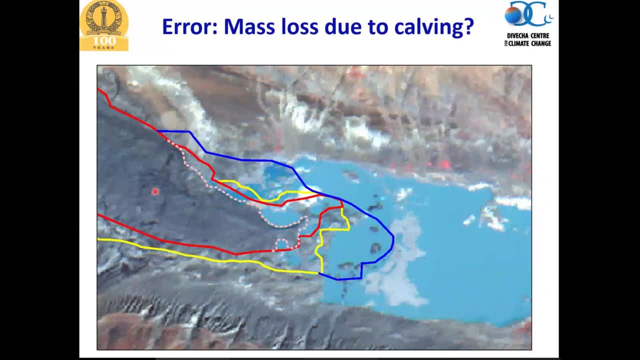 and pitch method making this is adding and pitch method making this is adding some error into the result. if there is some error into the result, if there is some error into the result, if there is a mass loss due to calming, so there are a mass loss due to calming, so there are. 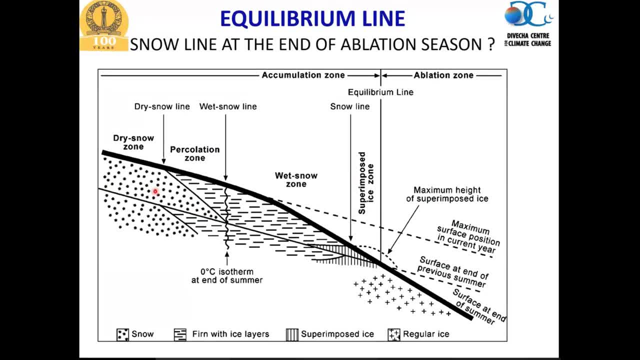 a mass loss due to calming. so there are- and you also know that- glaciological and you also know that glaciological and you also know that glaciological method is very demanding. that means you method is very demanding. that means you method is very demanding. that means you have to stay on the glacier for weeks. 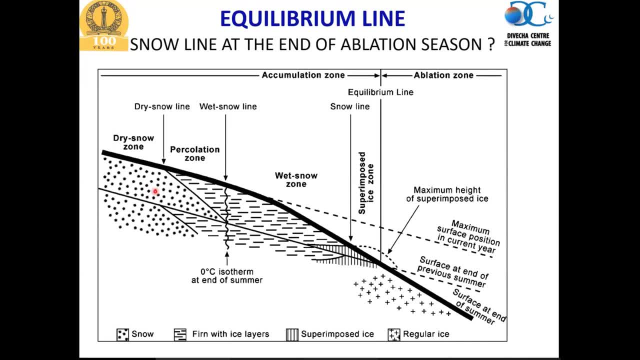 have to stay on the glacier for weeks, have to stay on the glacier for weeks and months and you require very large and months. and you require very large and months and you require very large infrastructure to support scientists on infrastructure, to support scientists on infrastructure, to support scientists on the glaciated height and bring them. 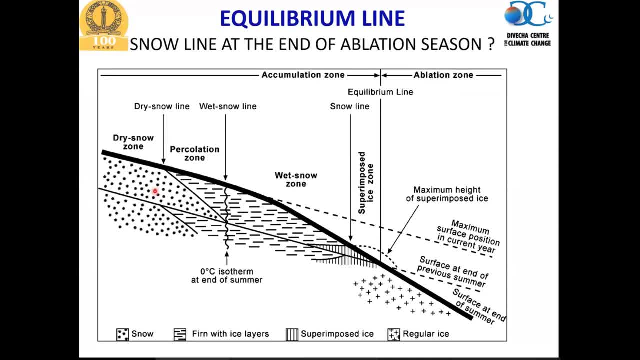 the glaciated height and bring them the glaciated height and bring them, bring them back safely on the ground. so bring them back safely on the ground, so bring them back safely on the ground. so, what you so as a result of this you, what you so as a result of this you. 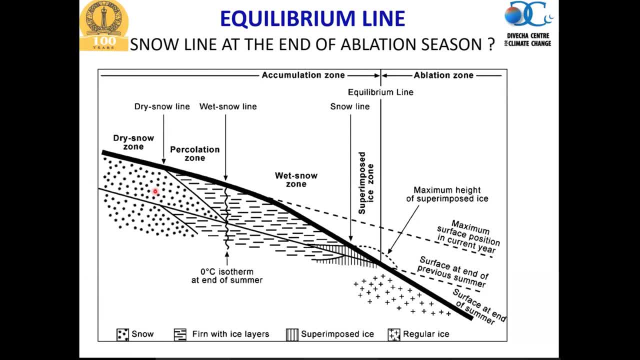 what you. so, as a result of this, you have a method which can be applied for, have a method which can be applied for, have a method which can be applied for very few glaciers on top of that, very few glaciers on top of that, very few glaciers on top of that. glaciological method cannot be applied. 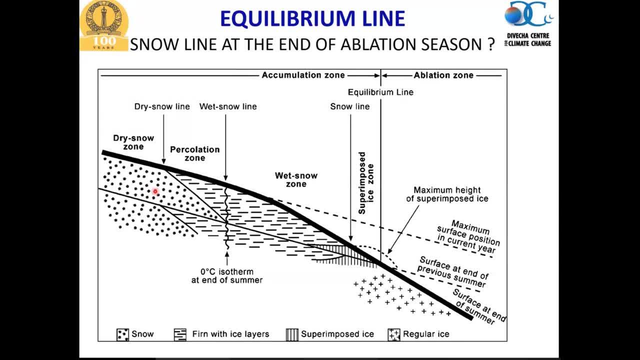 glaciological method cannot be applied. glaciological method cannot be applied for large glaciers because you have not for large glaciers, because you have not for large glaciers, because you have not in position to have. suppose you take the, in position to have, suppose you take the. 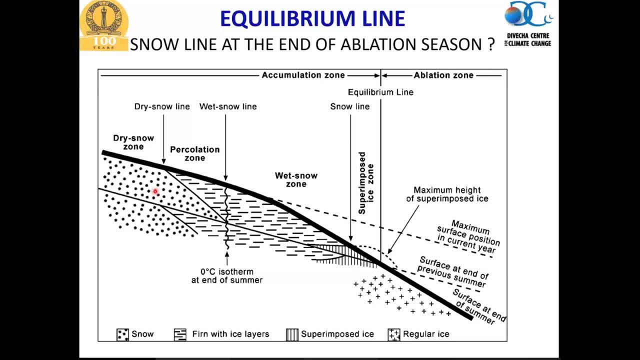 in position to have. suppose you take the Gangotri glacier, which is more than 100 Gangotri glacier, which is more than 100 Gangotri glacier, which is more than 100 square kilometer area, and you might square kilometer area, and you might. 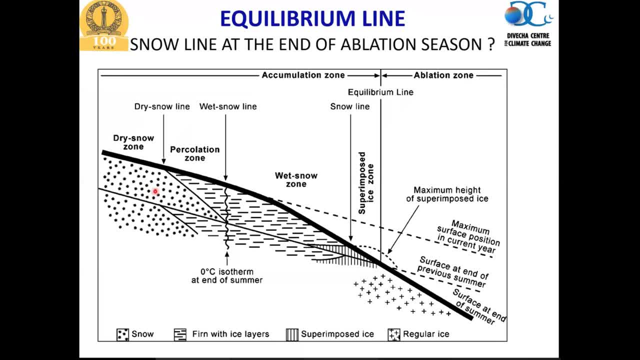 square kilometer area and you might read a thousands of state. of course you read a thousands of state. of course you read a thousands of state. of course you are not positioned to have that stakes, are not positioned to have that stakes, are not positioned to have that stakes and measure it. 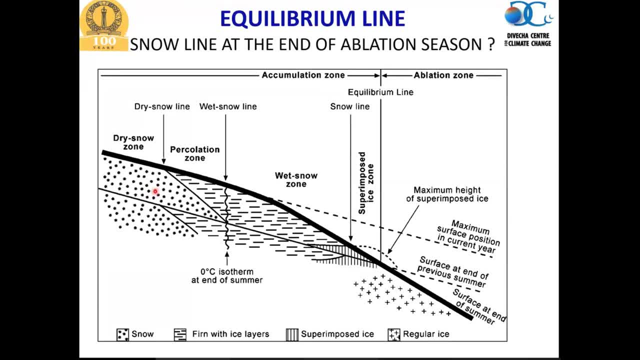 and measure it and measure it. so you tend to take a small glacier. it so you tend to take a small glacier. it so you tend to take a small glacier. it is four, five square kilometer in size. is four, five square kilometer in size. is four, five square kilometer in size. you tend to take it near the uh, near. 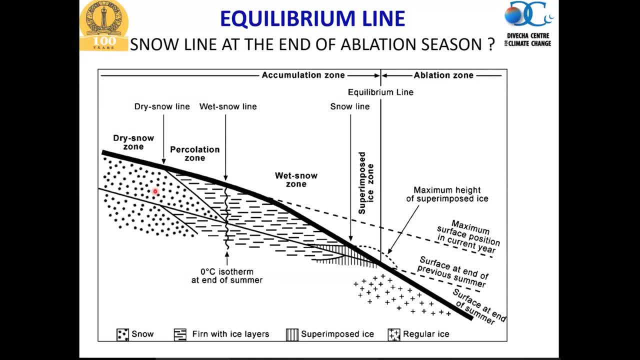 you tend to take it near the uh, near. you tend to take it near the uh, near the roadhead where you can. you quickly the roadhead where you can, you quickly the roadhead where you can, you quickly go and come back. so this creates the go and come back. so this creates the. 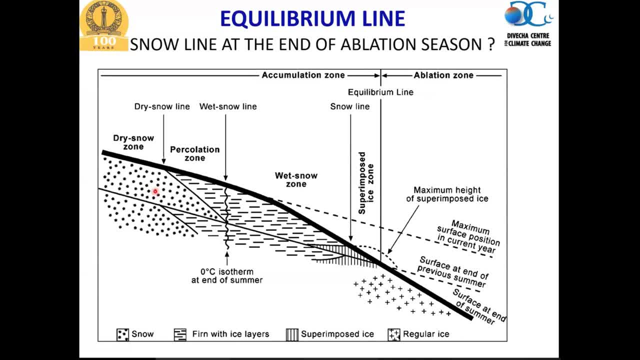 go and come back. so this creates the biased information about the glacial, biased information about the glacial biased information about the glacial health. therefore, there are numerous health. therefore, there are numerous health. therefore, there are numerous techniques have been developed. now to techniques have been developed, now to: 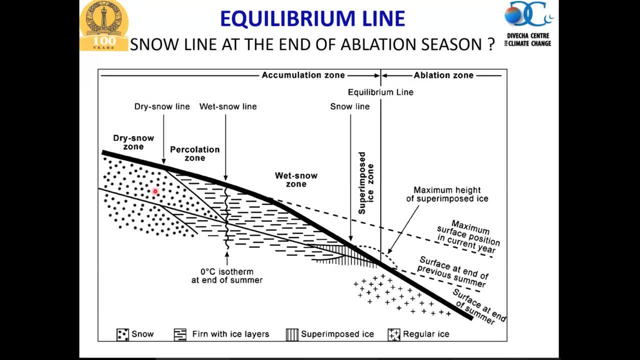 techniques have been developed now to estimate the mass balance, estimate the mass balance, estimate the mass balance, and one of such technique which is, and one of such technique which is, and one of such technique which is extensively developed, extensively developed, extensively developed, um, um, um by me, or a. 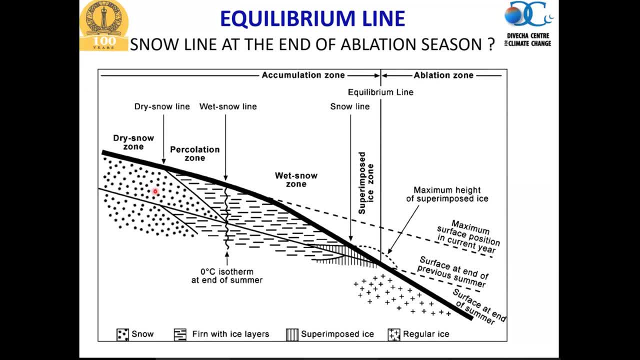 by me or a by me or a over a period of lot 20- 25 years, and it over a period of lot 20- 25 years, and it over a period of lot 20- 25 years, and it is now commonly using the equilibrium is now commonly using the equilibrium. 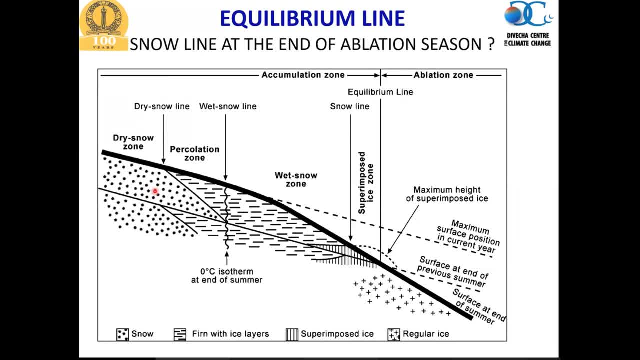 is now commonly using the equilibrium line altitude method, line altitude method, line altitude method. so so, so, we will look into this uh, this method. we will look into this, uh, this method. we will look into this, uh, this method. uh, but let us understand, uh, but let us understand. 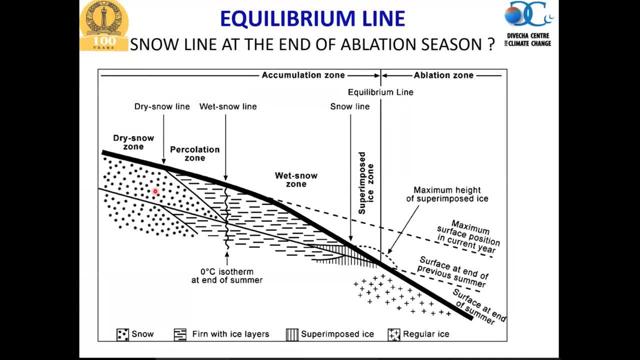 uh, but let us understand. what is the sign, scientific principle behind this method, so behind this method, so behind this method. so first understand the glaciers glacier, first understand the glaciers glacier, first understand the glaciers glacier, what it is and what it is and what it is and glacial surface. so 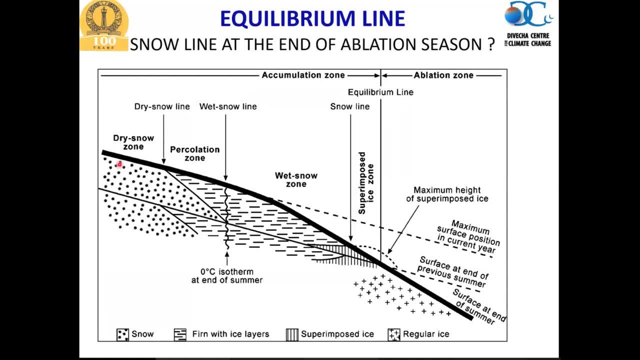 glacial surface. so glacial surface. so if we are in very uh high altitude, if we are in very uh high altitude, if we are in very uh high altitude, regions are in a. regions are in a. regions are in a, in a region where ci chain you go up to, 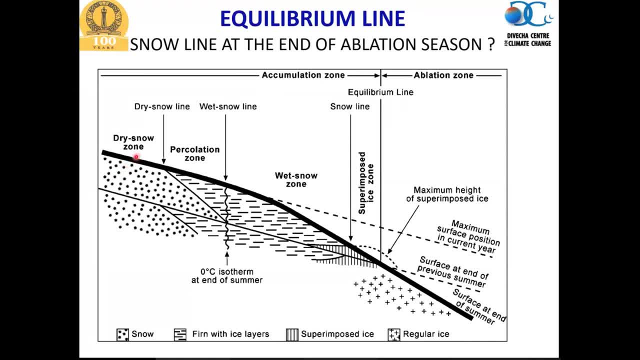 in a region where ci chain you go up to, in a region where ci chain you go up to six thousand, about seven thousand meter, six thousand, about seven thousand meter, six thousand, about seven thousand meter, after you go to mount everest region. after you go to mount everest region, 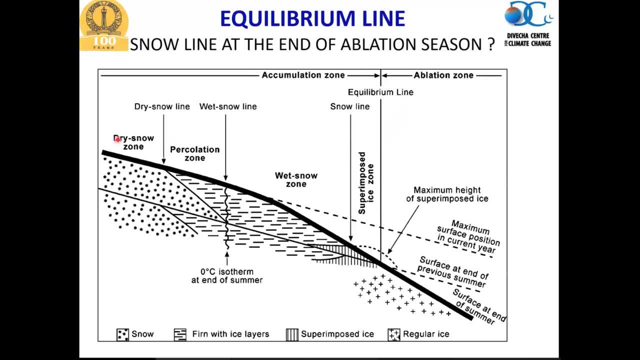 after you go to mount everest region, then there is that is called a dry zone. then there is that is called a dry zone. then there is that is called a dry zone region. that means in this region. region. that means in this region. region, that means in this region. there is no. 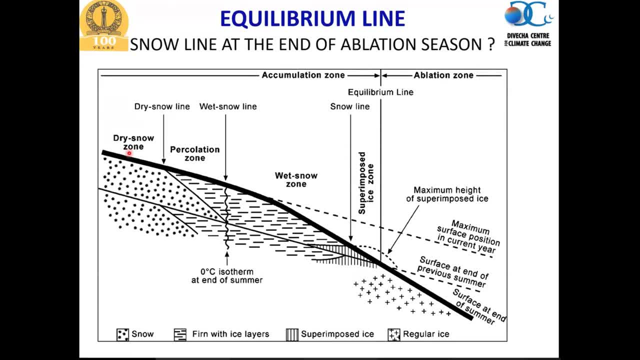 there is no. there is no. melting of snow takes place, correct. that melting of snow takes place, correct. that melting of snow takes place, correct. that is why it is called. is why it is called. is why it is called so. in himalaya, there is hardly any dry. 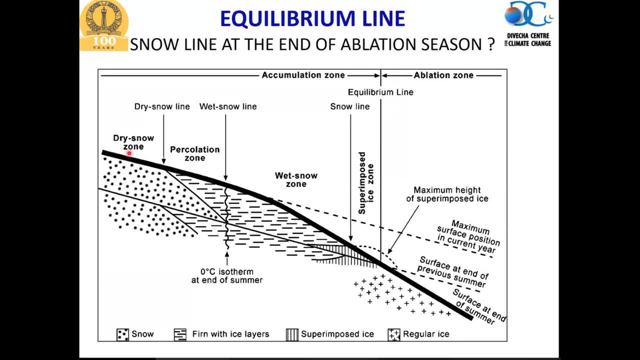 so in himalaya there is hardly any dry. so in himalaya there is hardly any dry snow zone. snow zone, snow zone- uh, it is predominantly dry snow zone. can uh, it is predominantly dry snow zone. can uh, it is predominantly dry snow zone. can seen in: 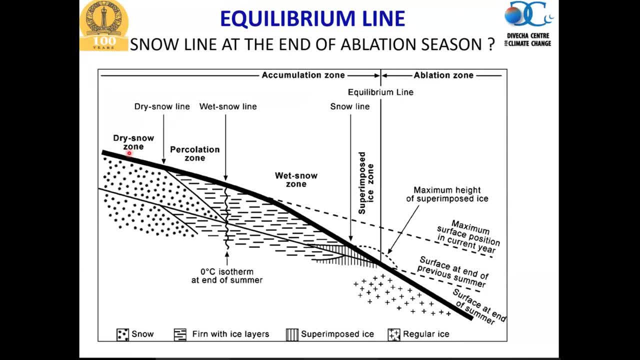 seen in, seen in antarctica and antarctica and antarctica and arctic region, arctic region, arctic region. then what happens is below that, there is, then what happens is below that there is. then what happens is below that, there is the percolation zone. 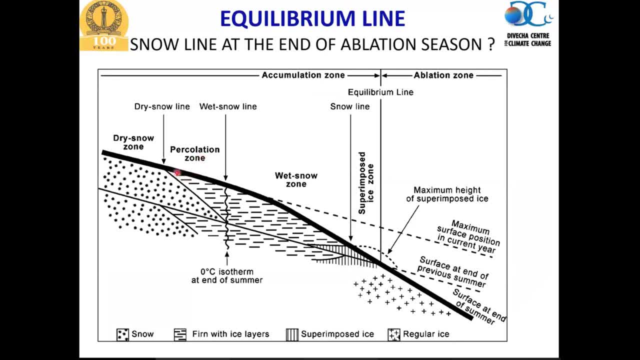 the percolation zone. the percolation zone, uh, what it means is, uh. what it means is: uh, what it means is: there is a sub melting on the surface. there is a sub melting on the surface. there is a sub melting on the surface takes place. 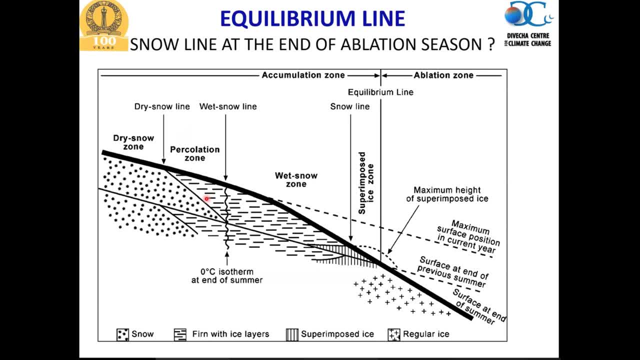 takes place, takes place. but that water which? but that water which? but that water which passes through the snowpack, refreezes it, passes through the snowpack, refreezes it passes through the snowpack, refreezes it again, again, again. and since it replaces, it increases its. 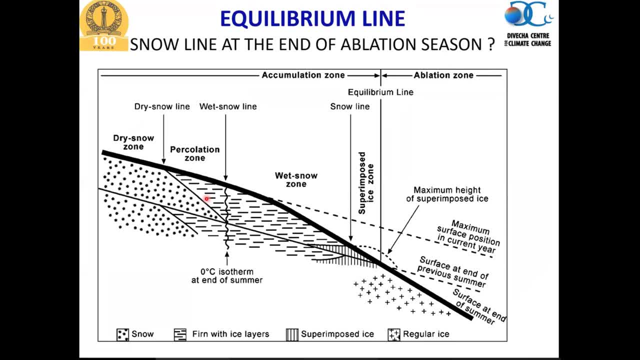 and since it replaces, it increases its and since it replaces, it increases its temperature, temperature, temperature. and because, and because, and because, when the refreezing is the exothermic, when the refreezing is the exothermic, when the refreezing is the exothermic reaction, and it, it increases the 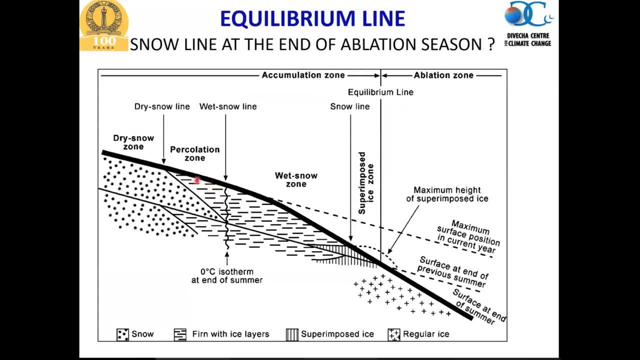 reaction and it it increases the reaction and it it increases the temperature of snowpack. so there is a temperature of snowpack, so there is a temperature of snowpack, so there is a so this, but entire melted so this, but entire melted. so this but entire melted melted water is consumed by snowpack. 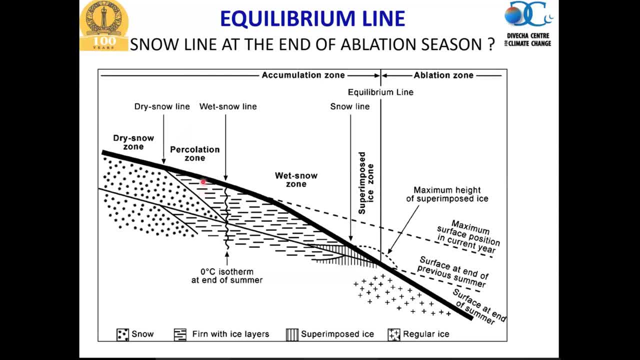 melted water is consumed by snowpack. melted water is consumed by snowpack to to increase its temperature, to to increase its temperature, to to increase its temperature. therefore, this is called a percolation. therefore, this is called a percolation. therefore, this is called a percolation zone. 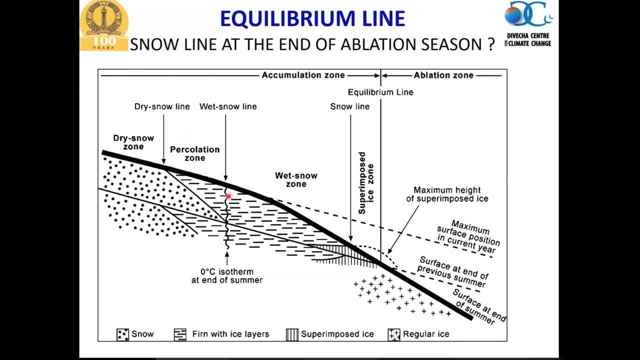 zone zone, but there is some point where, but there is some point where, but there is some point where, where there will be a water, which is where there will be a water, which is where there will be a water which is melted on surface, is reaches at the. 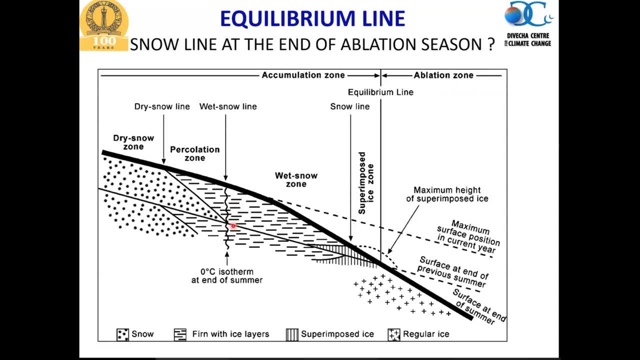 melted on surface is reaches at the melted on surface is reaches at the bottom or bottom, means at the at the bottom or bottom, means at the at the bottom or bottom means at the at the uh ice, uh ice pack, uh ice, uh ice pack, uh ice, uh ice pack. or i flow ice which is glacial ice, and 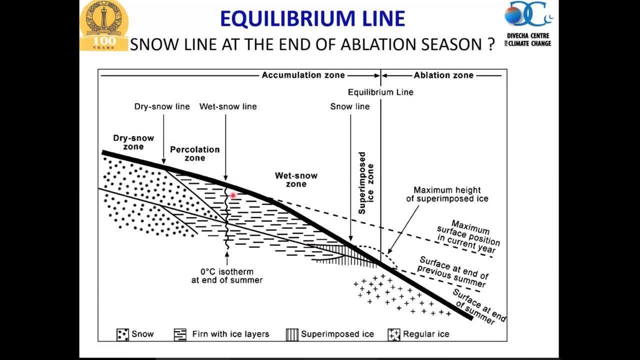 or i flow ice which is glacial ice and or i flow ice which is glacial ice, and entire this region, entire this region, entire this region, the snow region, converts into zero degree. the snow region converts into zero degree. the snow region converts into zero degree: isotherm. 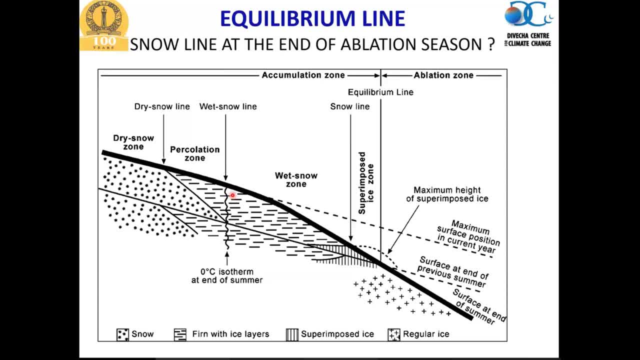 isotherm. isotherm, that means um, this is uh. that means um, this is uh. that means um, this is uh, because uh, here there is a melting snow, because uh, here there is a melting snow, and melting snow is at zero degrees celsius, so this developed, so this becomes a wet zone. 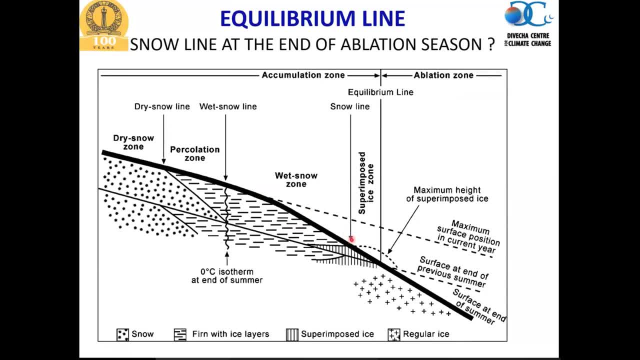 and then, as you come down, uh, then there is a line, uh, some, some, there is. there is a snow line. that means snow will end, that means the end of ablation area and then the accumulation area will start. then another thing happens is: uh, there will be a some region where superimposed ice will be there. 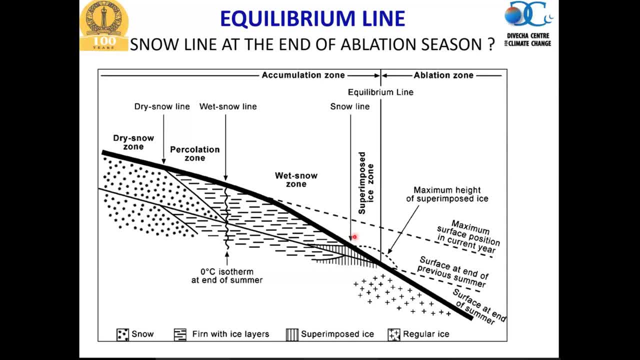 um, so what superimposed ice is nothing but, um, the snow is in process of converting into the ice, but some of that is very, uh, large chunks of snow or ice will be there in himalaya, because i have got many uh, i gone to the many glaciers in himalaya and i have gone to the uh, to the. 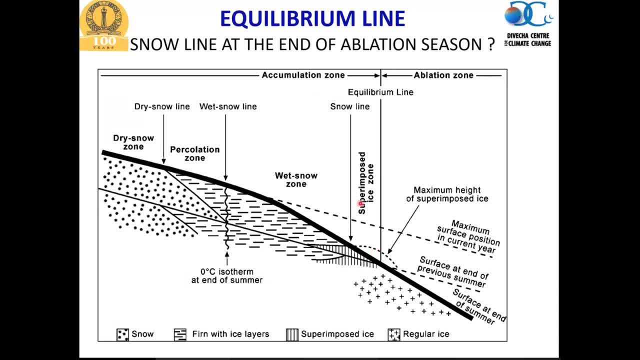 many glaciers in arctic. but in himalayas there is no superimposed ice, so it can line uh, which is at the end of a superimposed ice and from where glacier ice surface starts, gets shifted, so snow line becomes a, becomes a equilibrium line as far as himalaya is concerned. 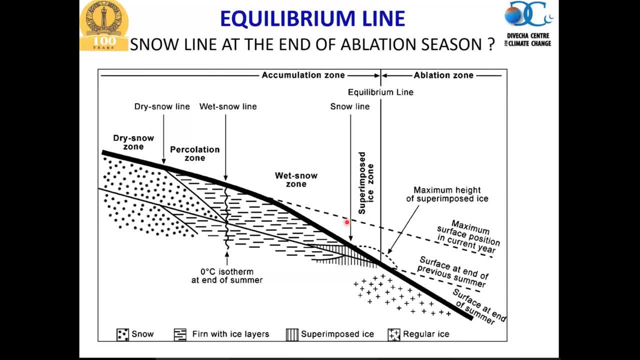 so that is how the importance of equilibrium line, so what it other way means is that is, if you can identify snow line uh into the himalayan glaciers and which is much easier to to uh, then uh, you can clearly identify the equilibrium line on the glacier. 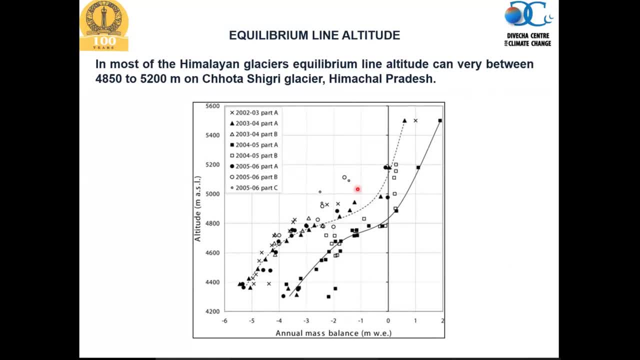 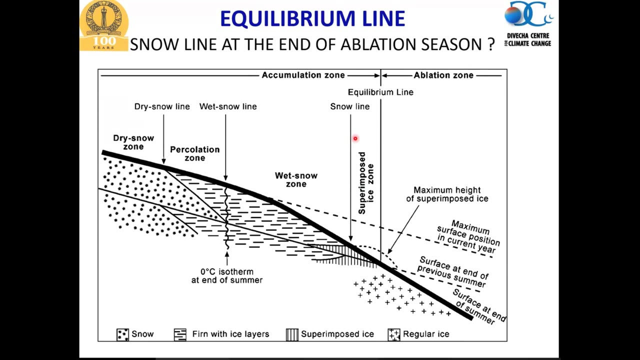 but what is this characteristic? how do you do it? uh, that, but there is another way of looking at the equilibrium line. this is one way of looking at the equilibrium. so what it means? it means if you apply, if you apply this principle, you know it means that, uh, 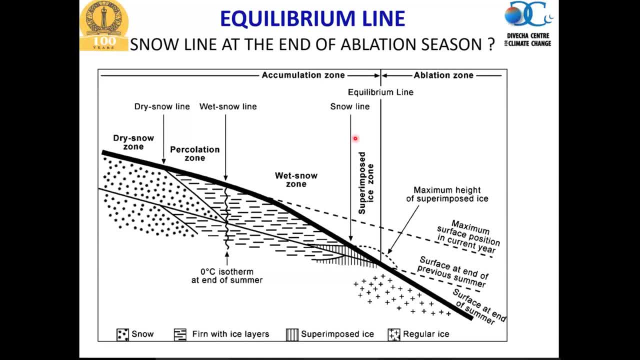 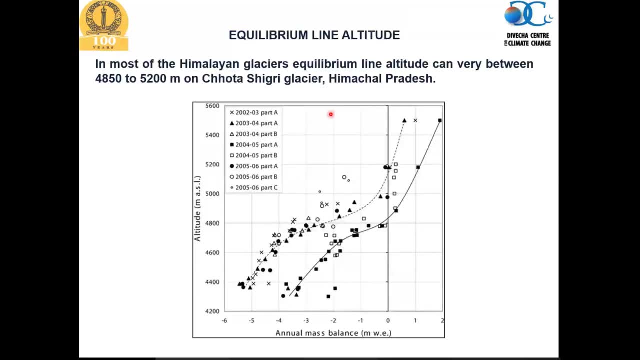 it means that the snow line which is at the end of- uh, if you can identify snow line at the end of summer, then this becomes a equilibrium line. that is the idea, but there are other ways which people have tried to interpret or estimate the snow line. uh, it means, if you plot a mass balance, annual mass. 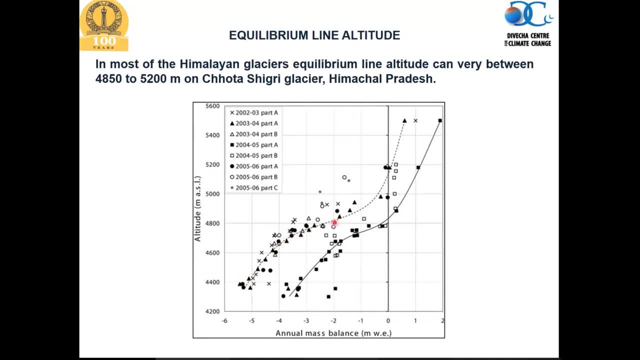 balance versus altitude and you plot the graph like this: wherever it cuts into into the zero mass balance, then it becomes the equilibrium line. so this is the equilibrium line. so this altitude: some year you have equilibrium lying about 5000, slightly less than 5200. some year you can have 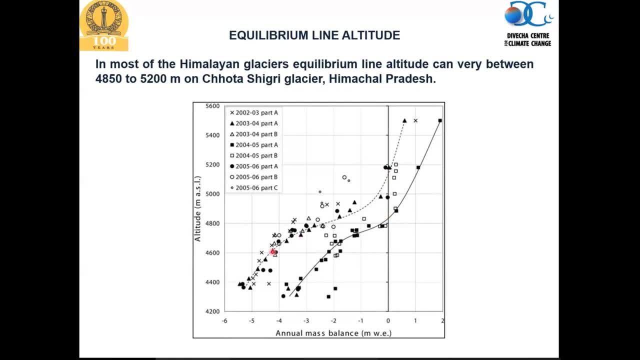 equilibrium line slightly above 4800. so this is how you can do if you have a glaciological method. so essentially now you have two definition of equilibrium line: altitude, one definition which, which is done by conventionally, where you, where you estimate the mass balance, and then 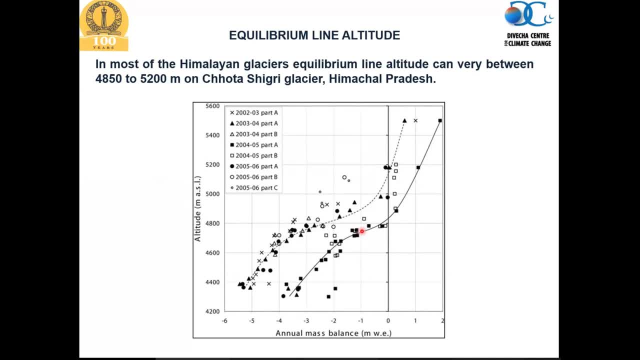 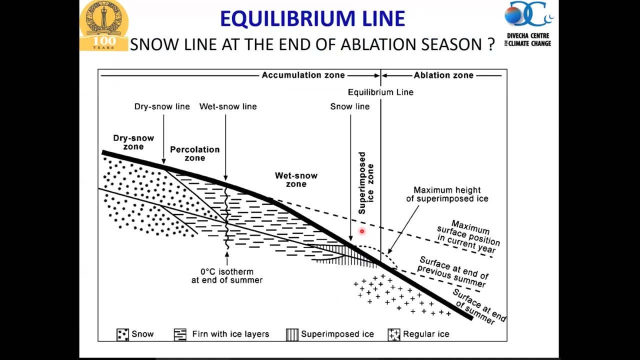 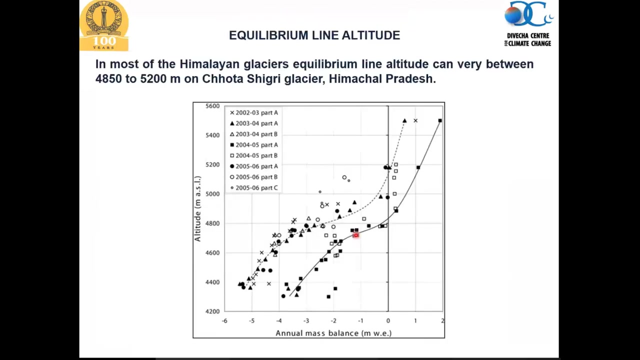 the mass balance. representing zero, um, representing the zero mass balance, is a, is a equilibrium line. however, this equilibrium line could be a we may not, may not be able to identify on satellite images, but this equilibrium line, where, where snow line represents uh equilibrium line, is possible for us to delineate like images. so this is how, way back in 90s, 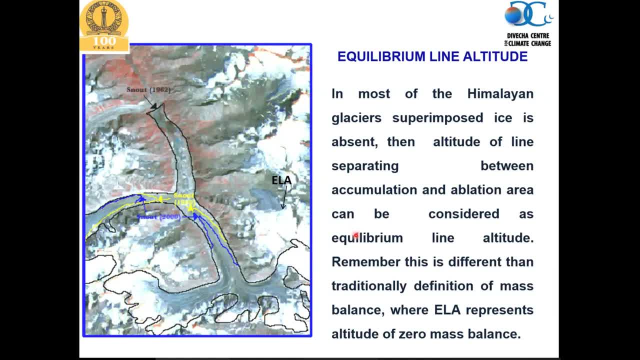 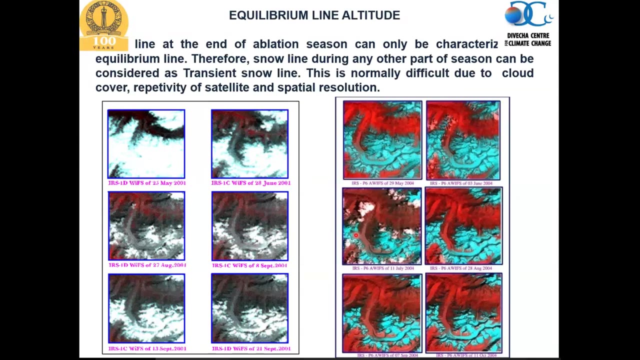 we have interpreted snow line and equilibrium line, and then that was um, that was really accepted and some of the- uh, some of the high profile papers published in general of glacier, and many people still use this definition to estimate the snow line and mass balance. so, having said that, how do you estimate the equilibrium line? altitude: it is a. 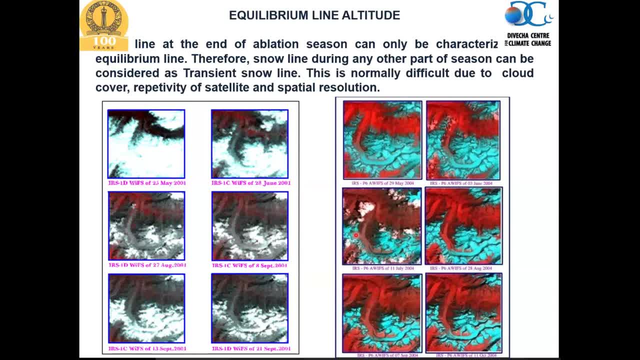 snow line. so as summer progresses, snow will start melting. you can see here: 2001. as summer progresses, snow line will start melting and ice will be exposed on the surface. you can see here: ice is exposed on the surface. ice will be exposed on the surface and. 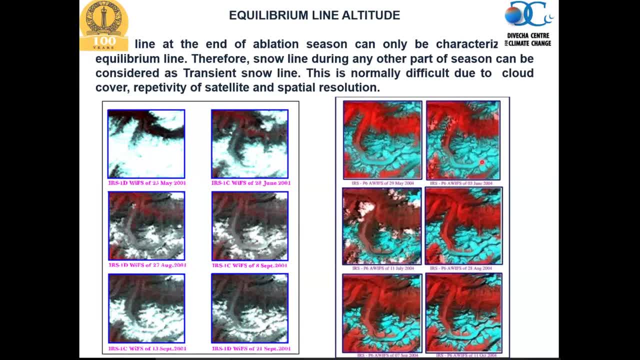 if world is ideal, this should go on retreating backward, this should go on requesting back, backward and it should retreat to the end of 30th september and you are able to get the mass balance, the position of snow line, and you have mass balance which is estimated by conventional method. 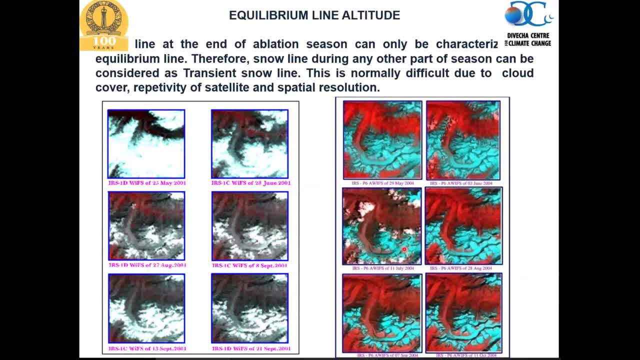 which is the 30th september. you correlate it and you get the mass balance. that is the original idea. however, you can see uh into this data and you will see that this is a whips data and this is a whips data. it it has around uh 56 meter resolution. it has around 60 meters. 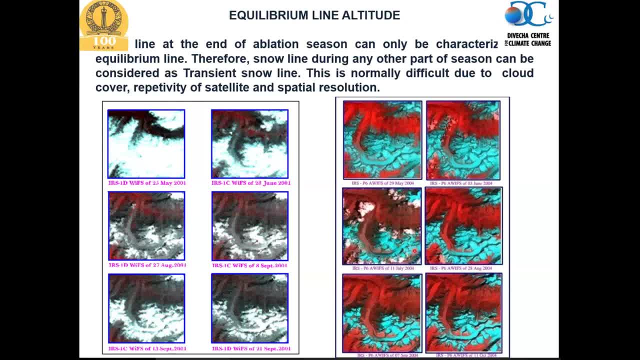 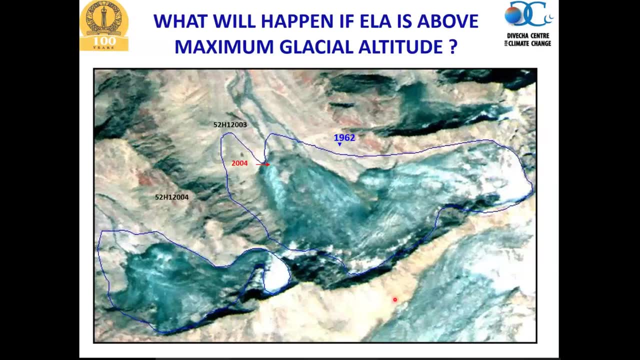 resolution and you can see that in 20th august. so it is uh, this. you may not get all the time. satellite images, uh, which is uh, which is a which can provide you good estimate. then another issue in this is what will happen to ela if, uh, uh, if el is above the maximum glacial? 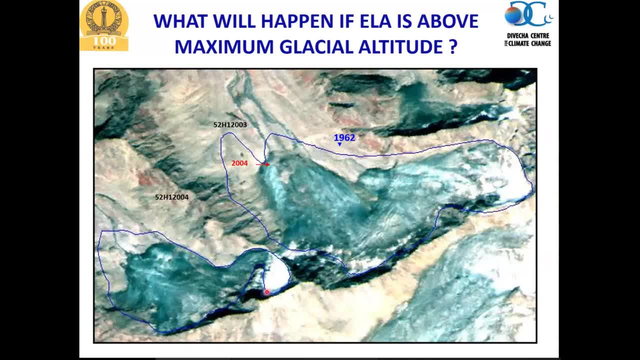 altitude. what it means is- you can see into this picture, except this small region, and here it is mostly- it is the cloudy. there is no snow on the glacier. that means entire snowpack is melted away and there is a. there is a ice which is exposed on the surface and therefore 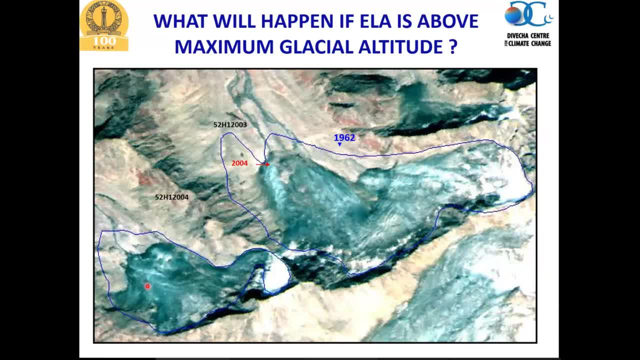 it is uh. now you have a position where there is there is no area above the line, And that means there is no accumulation area and glaciers are not in position to form a new ice, And this leads to the decapitation or terminal retreat of the glaciers. 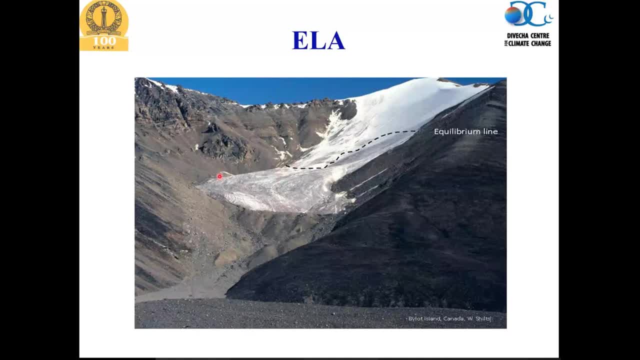 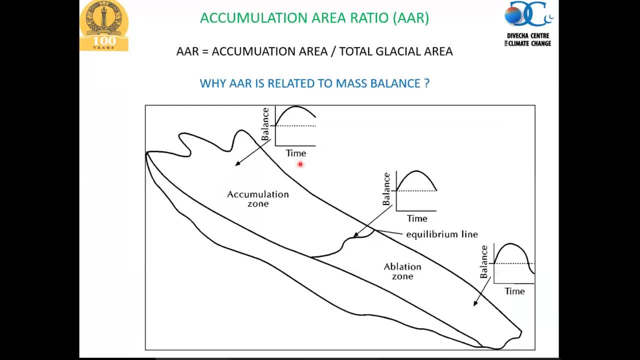 So how it looks like earlier you can see. this is that this is the ice and this is the snow, And you can see how how equilibrium line looks like. on on on this. So once you have a equilibrium line, then you can convert this equilibrium line, by using glacial area, into accumulation area ratio. 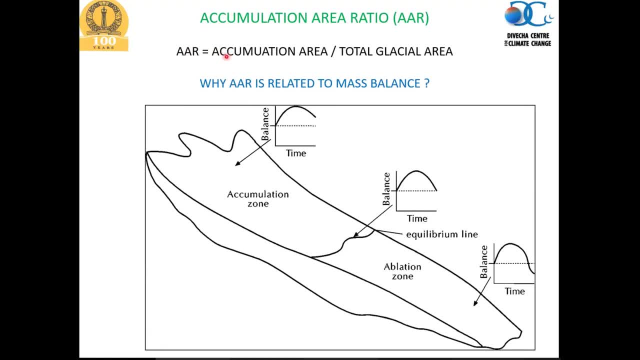 So accumulation area ratio is a ratio between accumulation area to total glacial area. So why air is related to mass balance is a very important thing. So you can see here the accumulation area. This is with time, The more snow is accumulated. So this is how this is. 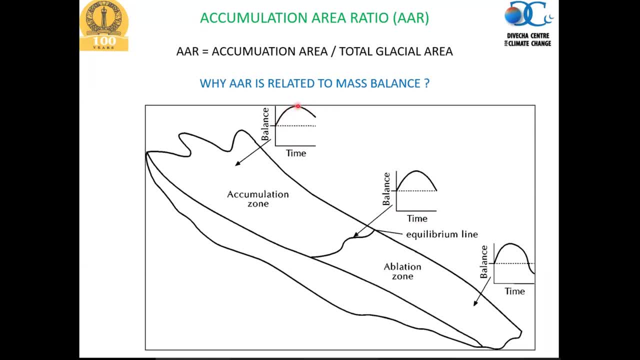 The curve will be time how it looks like It is more accumulated but it is melted less. So you have a certain amount of accumulation on equilibrium line. You have balance. That means amount of accumulation is equivalent to amount of ablation And in the ablation area you have accumulation and then you have. so you have total. ablation is higher than total. 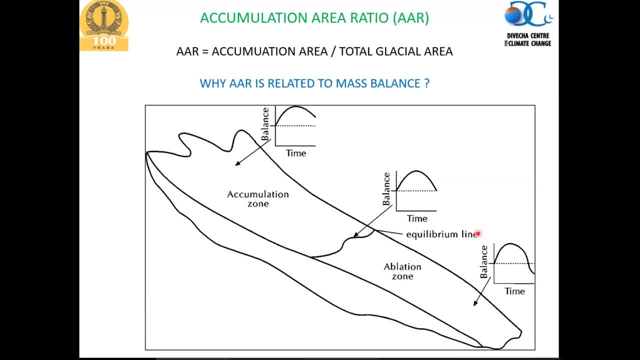 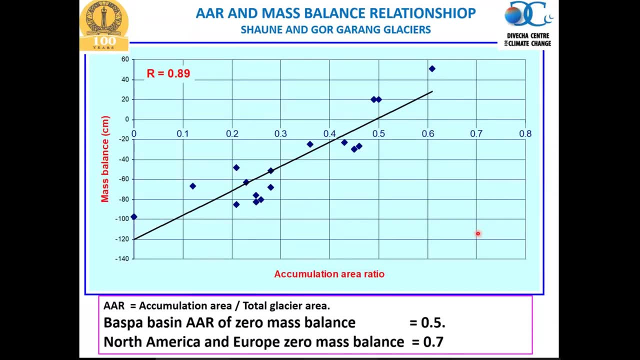 Accumulation. That is how they are linked with each other And therefore it is possible for us to do that. So if you convert air into mass balance, you require some relationship between the accumulation area ratio and mass balance. So if you are living in ideally idealistic world and remember, our mass balance is estimated on 30th of September. 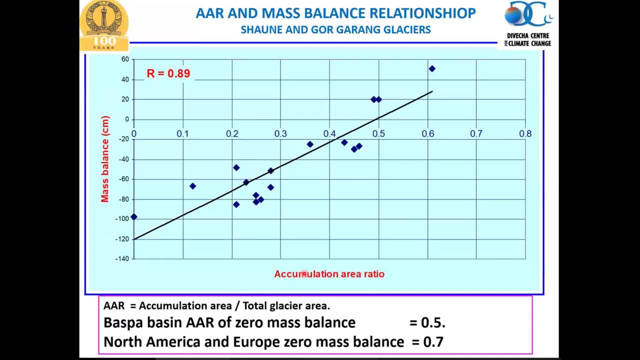 And if you have a satellite images which systematically gives you a retreat of snow line and you are able to detect the snow line at the end of summer, then you can plot, You can correlate this and get the mass loss idea. This method, You can advance the understanding. 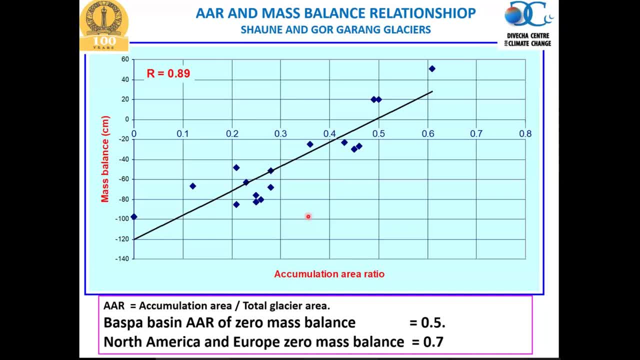 Himalayan cryosphere, essentially because until now this method was well developed in 1990.. And subsequently first paper was published in 1992 or 1993.. And then there are. there are numerous programs were launched, So first time we got glimpse into what is happening to glacier and large scale. 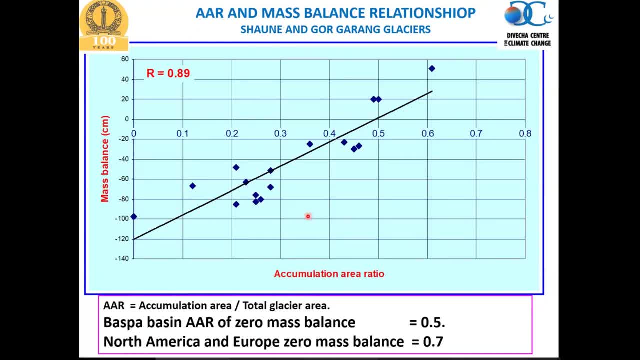 Until now, my balance was restricted to only one or two glaciers in entire Himalaya And people were trying to make some conclusion about that And, because of that, IPCC is 2007. confusion Came because of because of very limited data, data which is available for one or two glaciers. 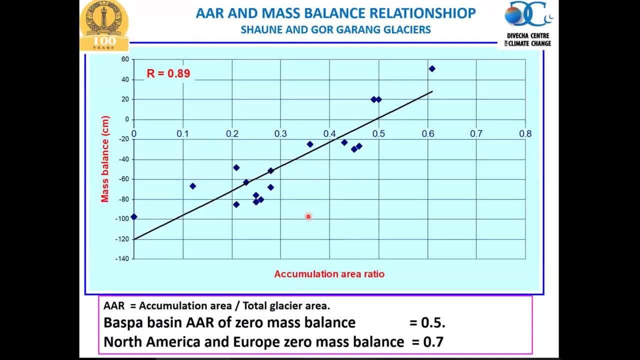 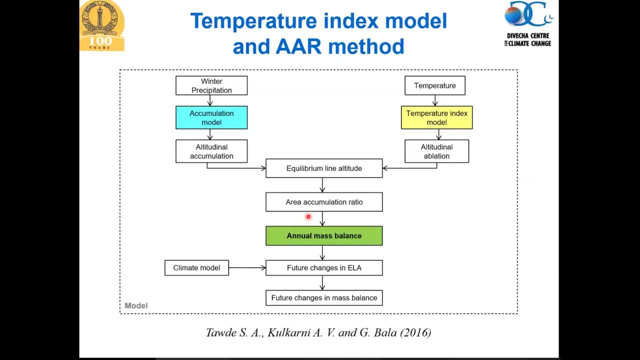 And they want to extrapolate for entire mountain range, and making mistake in doing that. But this technique, first time, has provided you opportunity to look into thousands of glaciers in one go and provide a smart balance. However, we know that that two things we know by now. 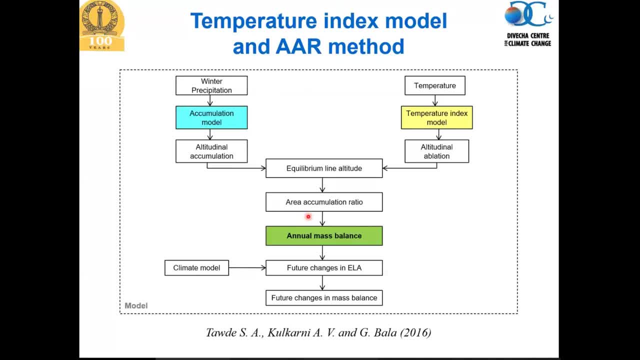 So one thing we know is all about we required a satellite images which is at the end of summer. end of summer, But there is some difference between the end of summer and the mass balance which is available in India. Indian mass balance is available 30th of September. 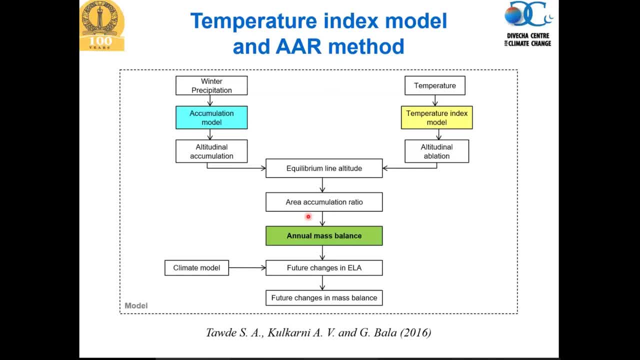 So end of summer did not be close with that. So it creates, creates it, And then, because of the cloud cover And because of the seasonal, unseasonal snowfall, you may not be able to get the snow line which is at the end of summer. 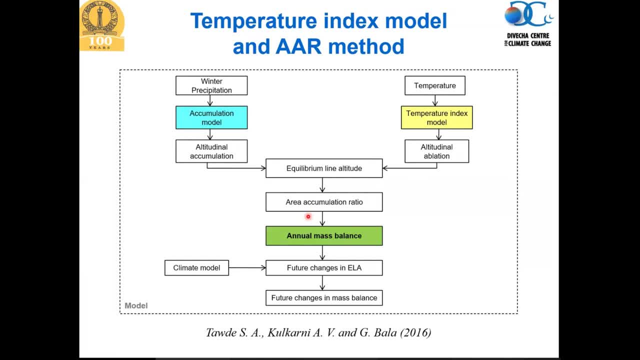 So what do you do now? So even the original technique was developed in mid 90s. You can see, subsequently, one of my doctor students had developed this technique where she had used two important ideas to improve it further. First thing is: We have winter precipitation and you estimated the accumulation model? 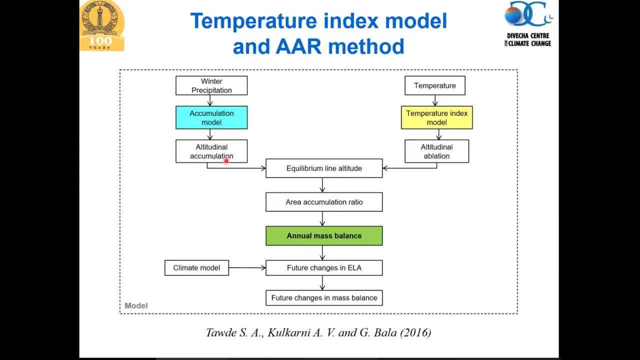 You estimated in each altitude zone how much is a snowfall or snow accumulation. You have a temperature, Then apply temperature index model and get ablation in each altitude zone. So once you have this, you, you, you validate it. For which? 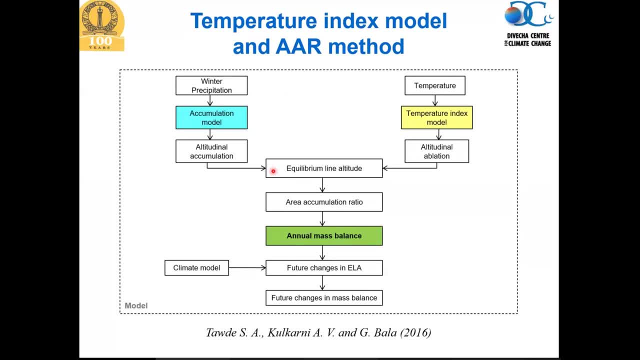 There is no for certain period of year where there is no snowfall, And and then you run it till the end of September and you get the imaginary equilibrium line of September And then from there you got the accumulation area ratio and you get the annual mass loss. 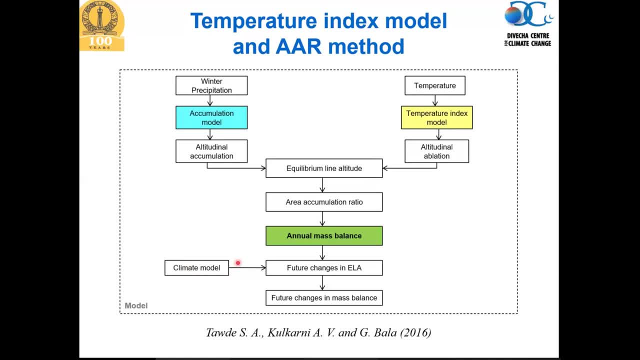 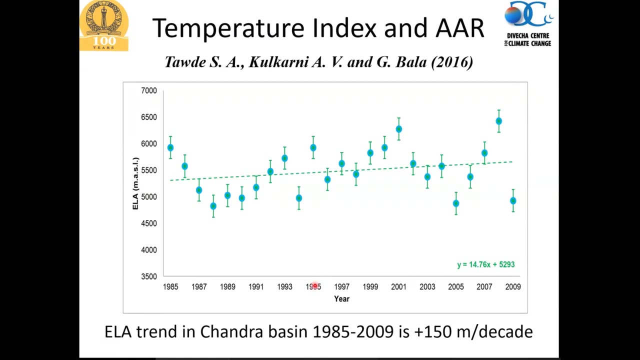 This model has the advantage because it can be forced with the climate models and it can give you future changes in ALA And future changes in mass loss. So this is a much better method to do it now And I'm sure some of you will do exercise on that. 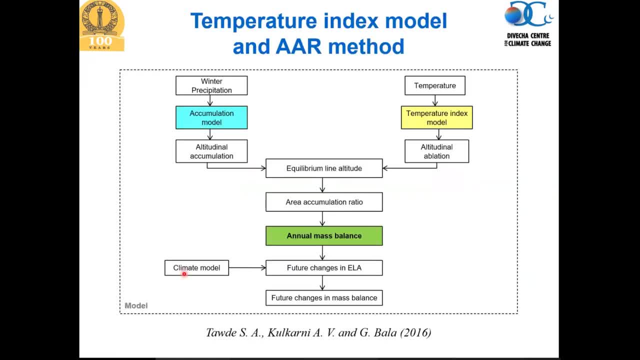 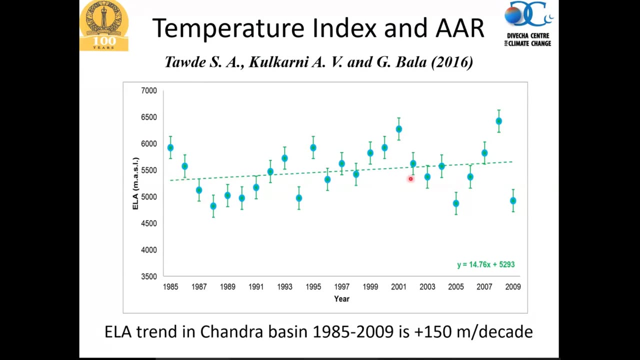 Advantage in this method is it is predominantly, if you look into that, it is predominantly based upon the temperature and precipitation And satellite data is going for the validation purpose. So you can run it for a period which you have a satellite, You have a temperature and precipitation data. 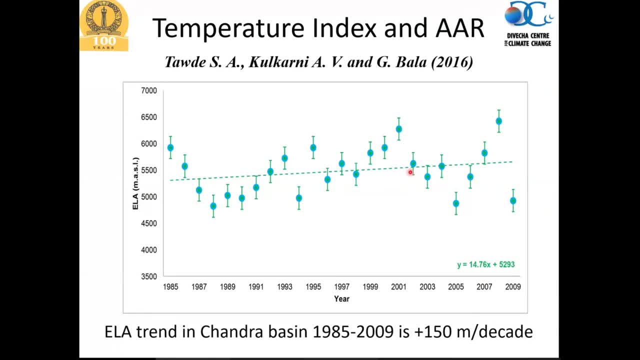 And it is quite possible that you have a large and you can do it annually. You can do hundreds of glaciers by by developing programs And this is how she has done it And she has estimated annual change in mass balance from 1985 to 2009.. 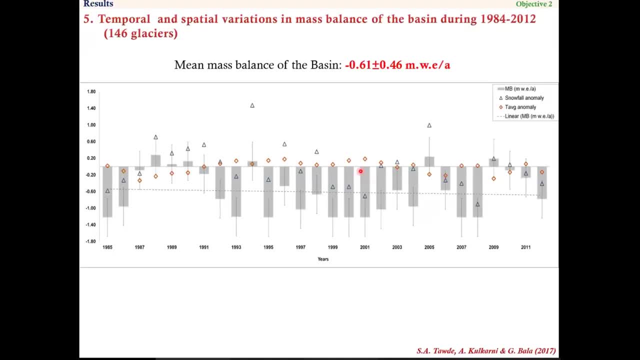 And this work was done. You can also have Special variability of snowfall, The Temporal special mass balance of basin during 85 to 2016.. You can, you can really really do that And you can also see for some year. 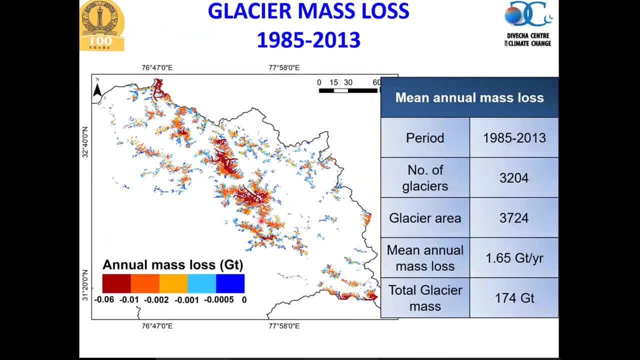 Mass balance is very negative some year, So you can understand the trend. You can also do the And you can see here The blue is showing very Relatively less Mass loss, Mass loss, But some, Some glaciers Are having. 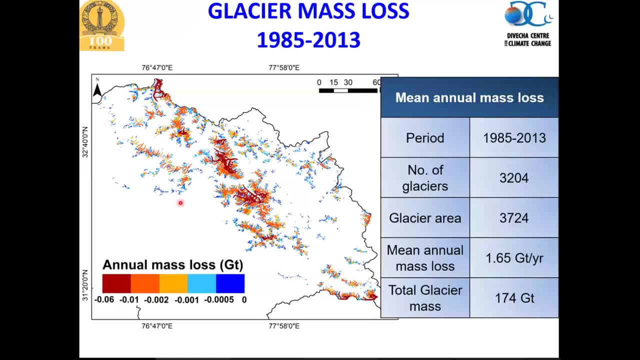 Very little Mass loss, But some glaciers Are having red tone is showing Very high Mass loss, Clearly suggesting that There's a special heterogeneity in mass loss And some Glacier. So It is, It is, It is. 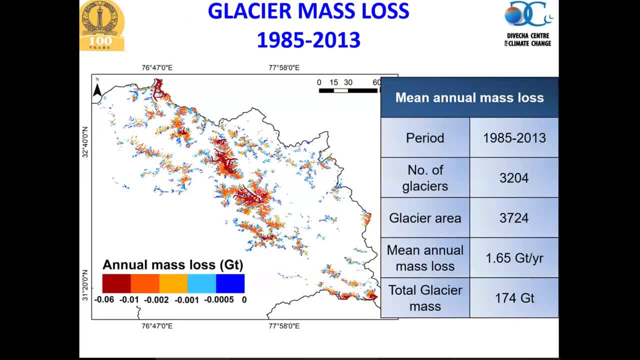 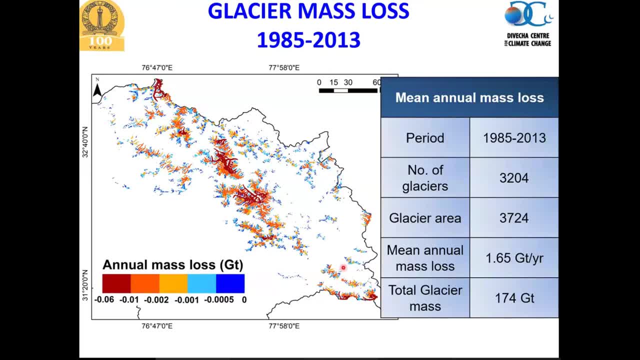 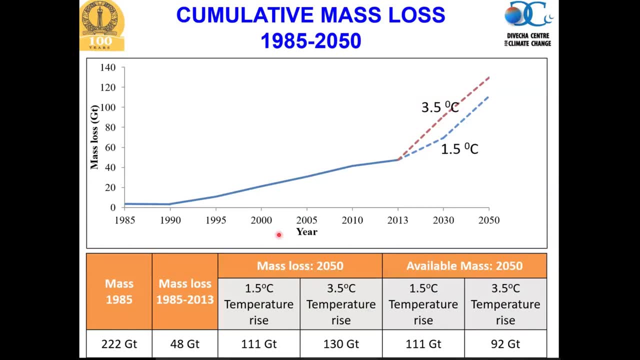 Glaciers to that located Low altitude region Are likely to face Um Are linked to the US Significant Mass loss. So We can Take that And we can understand How glaciers I'm going to lose. 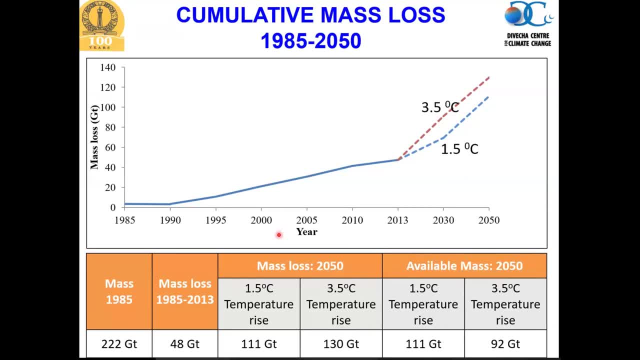 Yeah, We kind of Also plugged it Into the keyboard More dead. I say that how climate model is going to change in future, how temperature and precipitation are going to change in future And if you can some models suggest by middle of century. 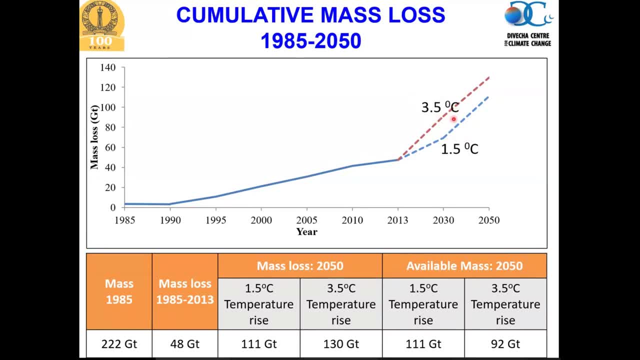 1.5 degree rise in temperature. some are saying 3.5. And then you can plug into the model and say how glacial mass loss is going to change in future, how it is going to accelerate in future. So all kinds of further analysis you can do. 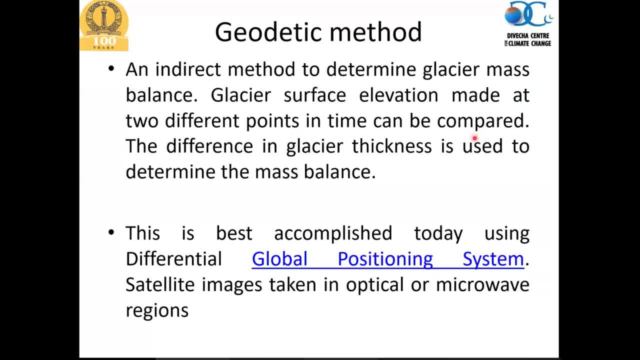 And I am sure some of you, these exercises we will do, you will do in today afternoon. There are another method to understand glacial mass balance is geodetic method. What this method is, this is an indirect method to determine glacial mass loss. 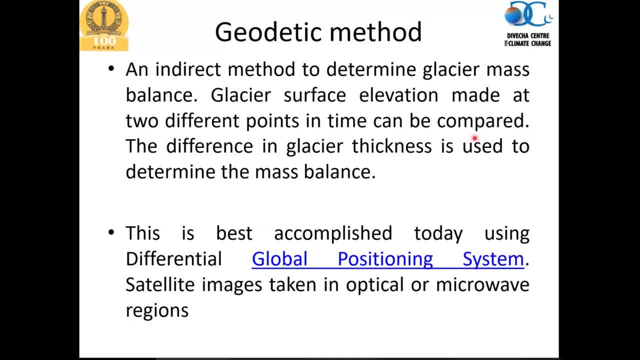 What essentially you do in this method is you develop a digital elevation model where you get the surface elevation of glaciers. After a couple of years or a few years, you again develop the DEM And then the difference by differencing the DEM, you get the glacial change in thickness. 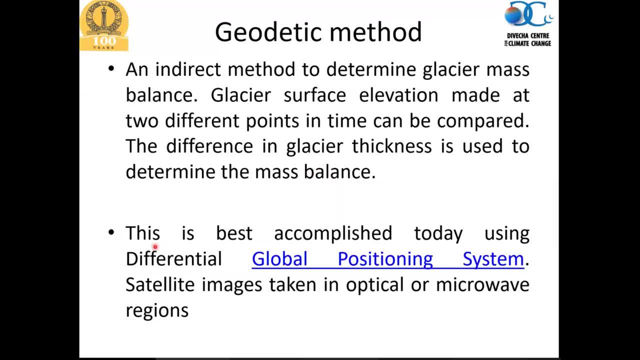 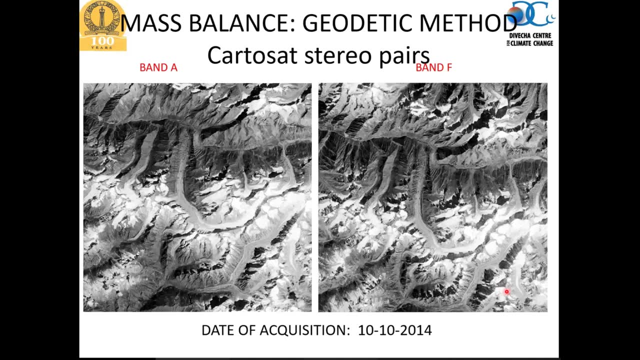 multiplied density and you will get the mass loss. So you can best accomplish by differential glacial GPS system or satellite taken by optical or micro region. can we do it? So this is the one satellite picture where you can estimate mass balance by geodetic method. 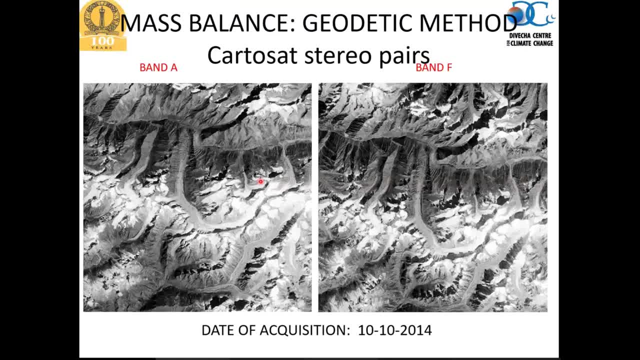 It is a cartosat satellite image and this is a on the two, one forward-looking and backward-looking camera on the same satellite, and you can take the two picture. when, when two pictures are there, you create certain model and then you get the parallax and by knowing parallax, 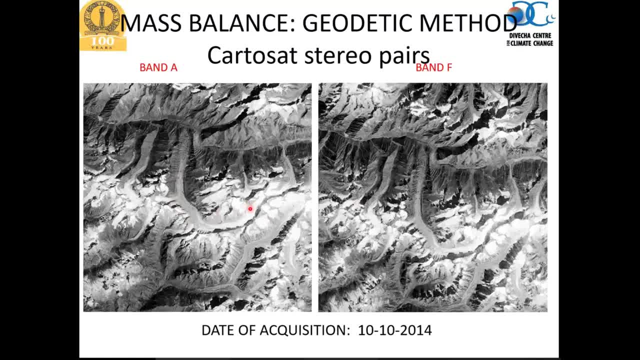 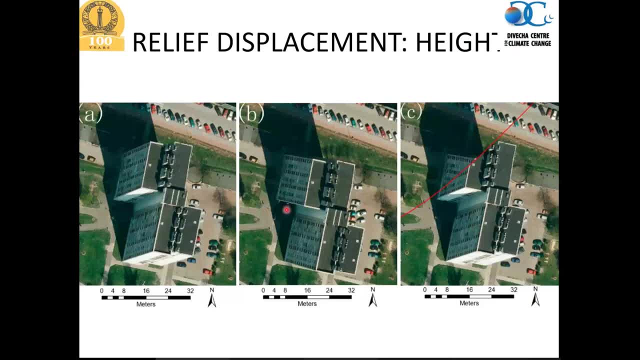 you can estimate the elevation, You can have a historical DEM, you can use the historical DEM or you can use So what it gives is a real placement. So you can see here on this picture is if photograph is taken exactly vertically down, then the bottom and top of the surface should be at same place and 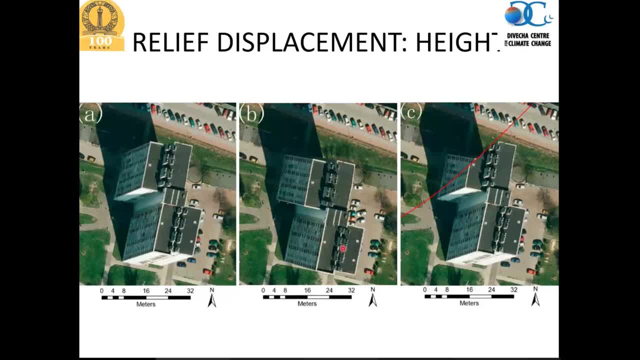 depending upon its shift. how much? this is this position? top is this position? both the position actually should have been on one spot, but they are not there because there is a shift. that is shift because satellite has taken picture by angle and it has created the parallax. 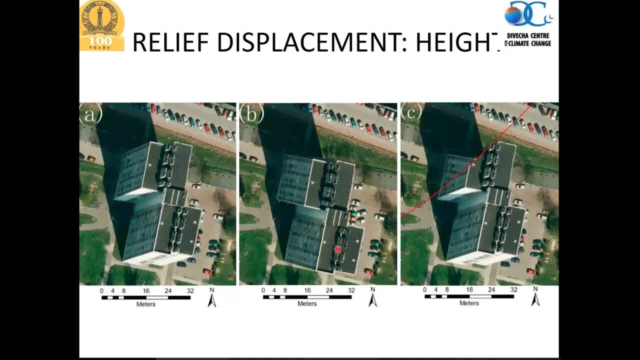 Now this parallax are you called it as the relief, displacement, using characteristics of the glaciers? for a characteristic of the of the sensor of satellite is altitude various. So one of the characteristics of the of the sensor of satellite is altitude various. you various other things. you can generate the DEM and you will do that. 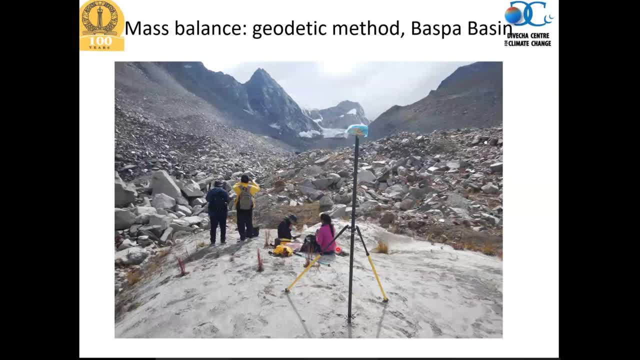 So you go into the field. If you want very accurate, then get the GPS points. the mass balance into this is one which we are done in in a bus by basin, where you go on into the field, collected the points and then use it in satellite images to estimate the change in elevation. 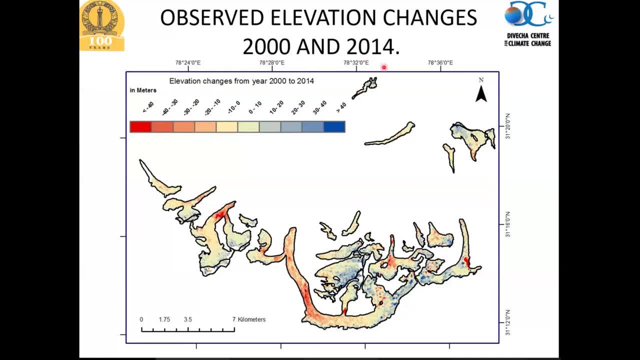 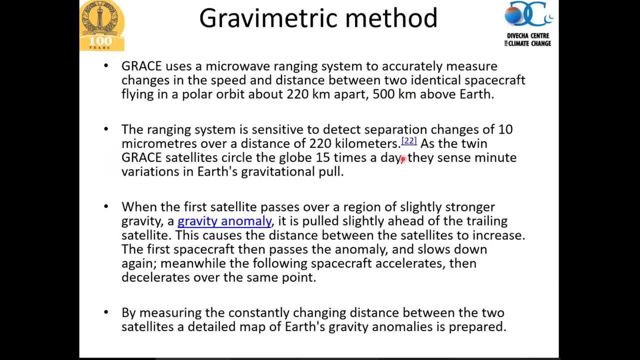 So you can see here observed elevation changes from 2000 to 2014.. How elevation is changing, you can say, and this will help you to get the mass balance. Another method to estimate the mass balance is called a gravimetric method, where the GRACE 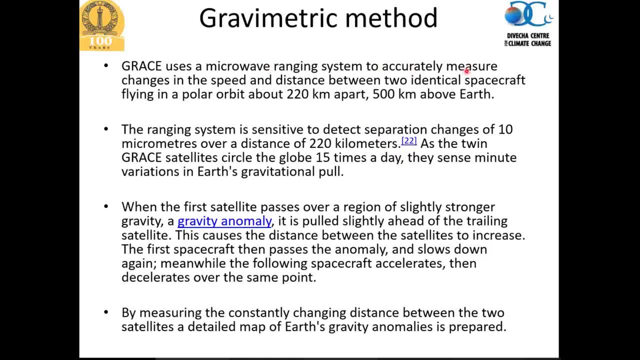 satellite uses the microwave. So what Essentially it is? It is The GRACE satellite is essentially measuring the gravitational pull or gravitational field of the earth And it has the two satellites, which is flying at around 220 kilometers and 500 kilometers above the earth. 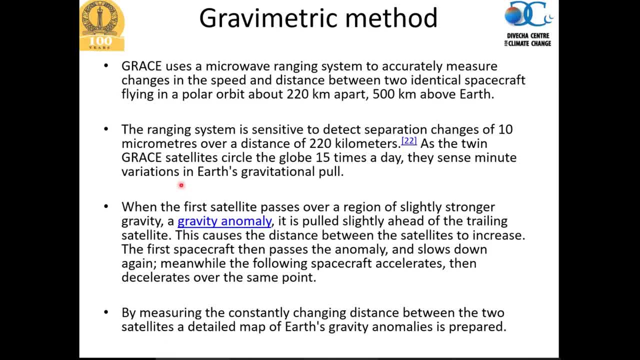 And when it comes to the, it comes to the places where and the separation as it moves through the on the surface of the earth. So, depending upon gravity, there is a minor perturbance which takes place and this minor perturbances are used to estimate gravity anomaly and that grade. 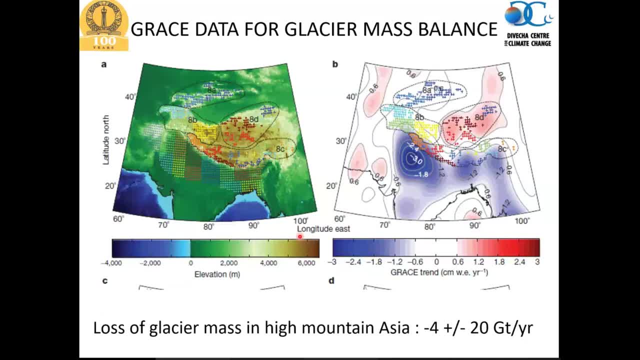 So it is used to estimate the change in glacial mass. There are still a lot of accuracy in this and you can see the greatest data of glacial mass loss. This is very high accuracy in high mountain Asia. But This is significantly now being and hopefully we will have better results. 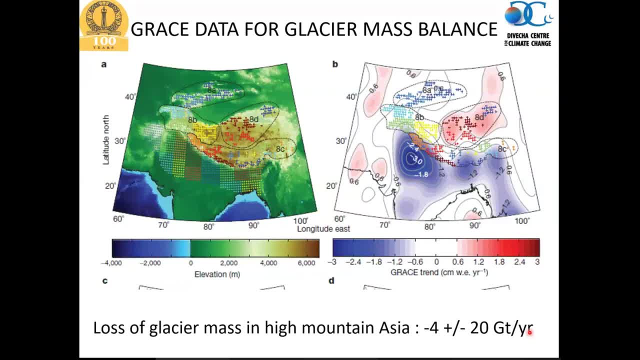 So what? Essentially, if you look into into the overall mass balance, you have a first method, which is a glacial logical method, which gives you more balance about individual glaciers. More people rely on this because you put a lot of effort in doing that and that you get. 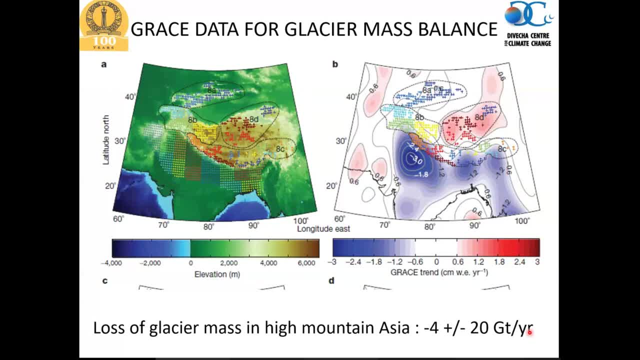 the small glacier. Yeah, And then you have the geodetic method, which is a geodetic method which, by using change in elevation, you can estimate my battle, and you have third, So these two make one method is for individual glaciers. 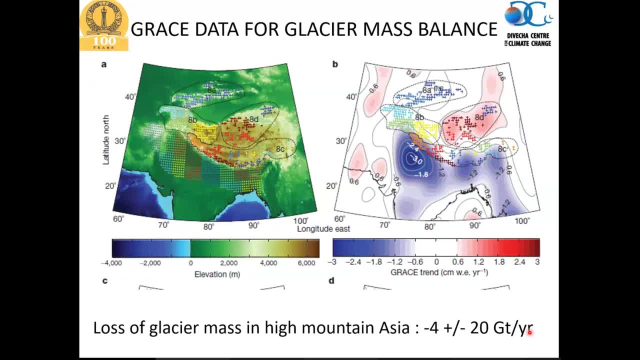 Geodetic method. you can do it for large geographical area and the grace method will give you estimate for entire mountain range. So you have. you can use this method in different spatial domain. Accumulation- Accumulation area ratio- will provide you information on individual glaciers also.